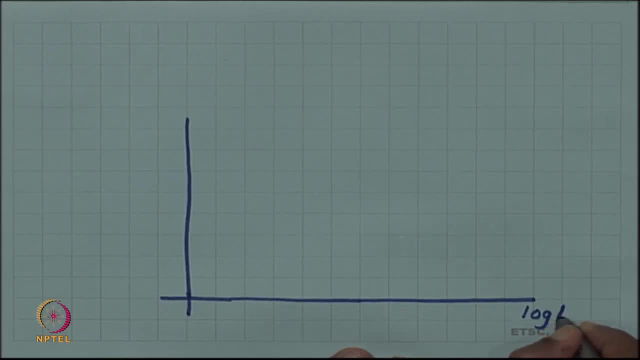 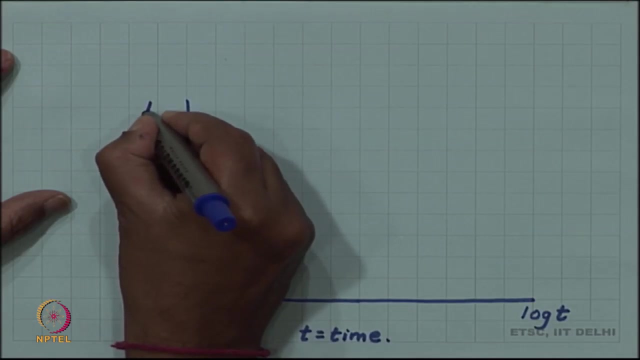 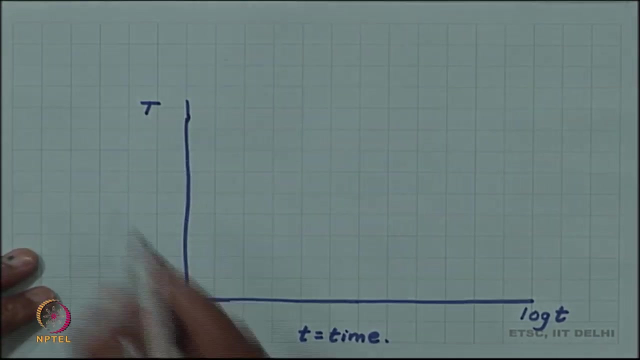 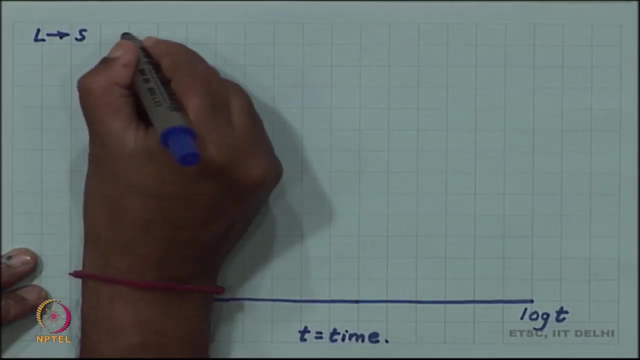 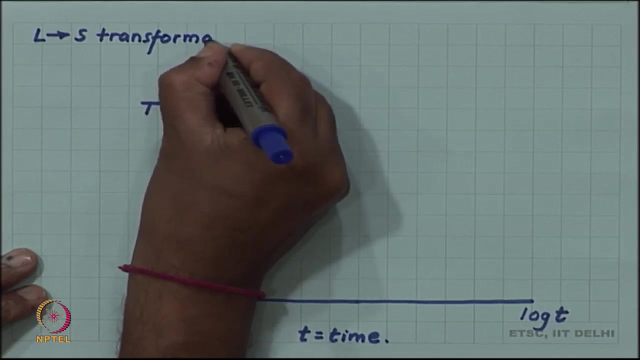 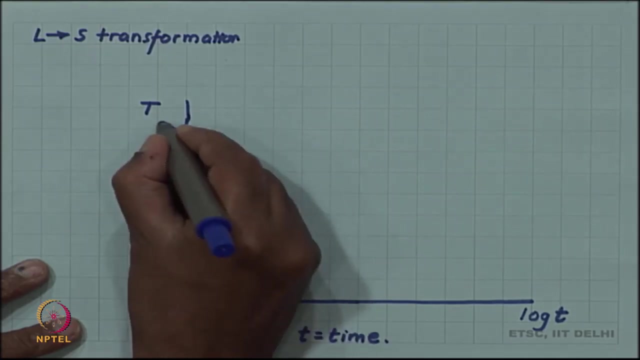 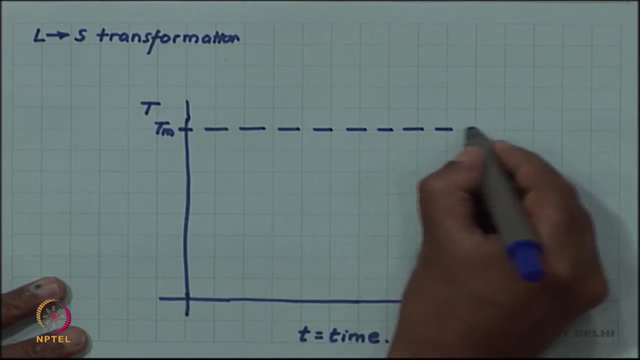 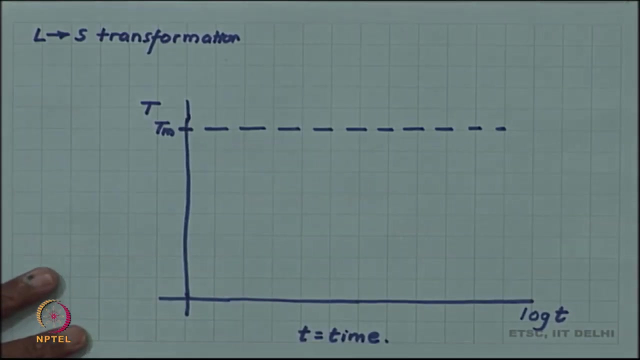 the time is given in logarithmic scale, So we have log t and here we have temperature. Again, let us look at as an example liquid to solid transformation. So we have critical temperature, which is the melting temperature above which no transformation will happen. So we can draw that line and we have already seen that how the transformation 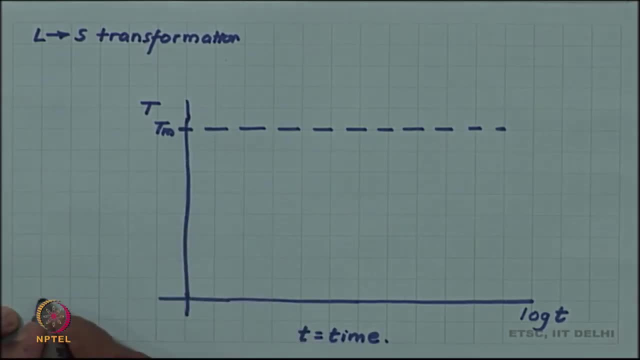 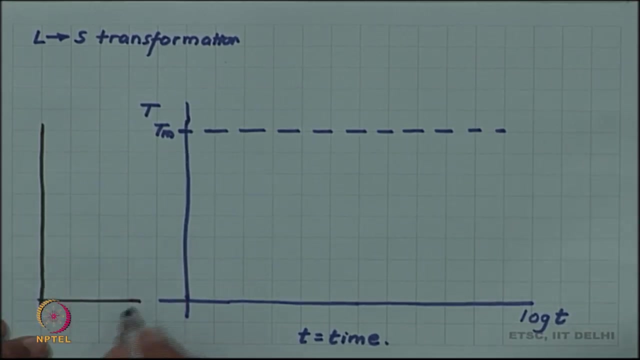 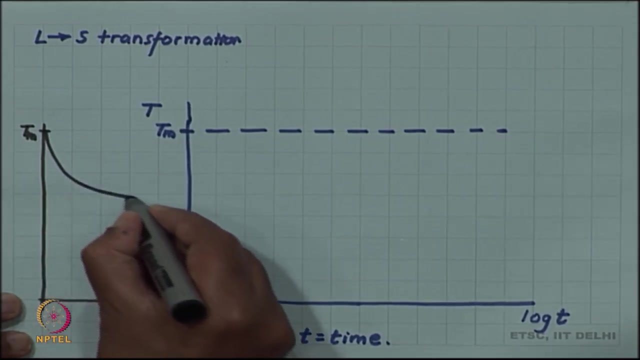 rates change as a function of temperature. So we can build that diagram here. Recall that we saw that at melting, as a function of temperature, the overall transformation rate goes through a maximum, it goes through a maximum, it goes through a maximum. So 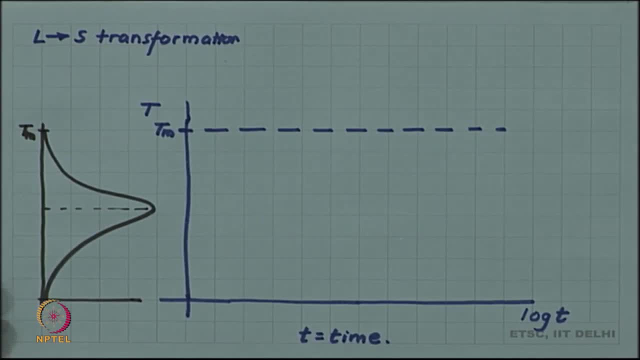 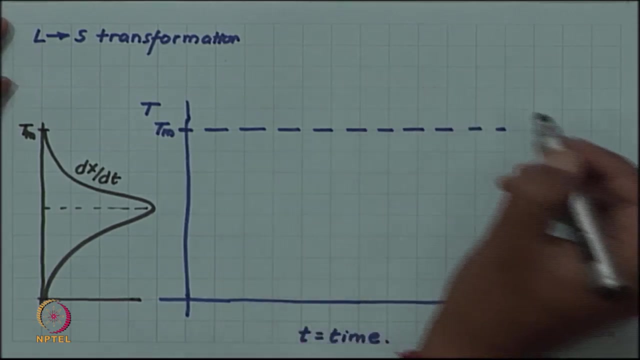 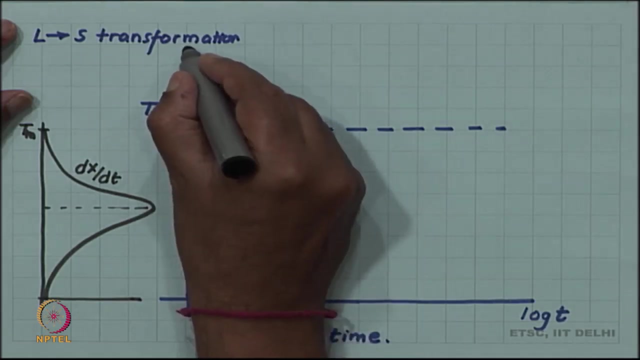 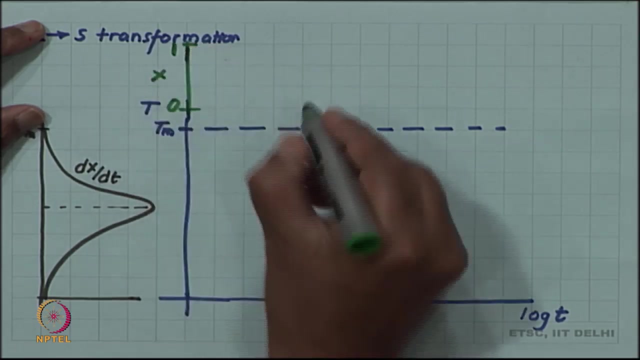 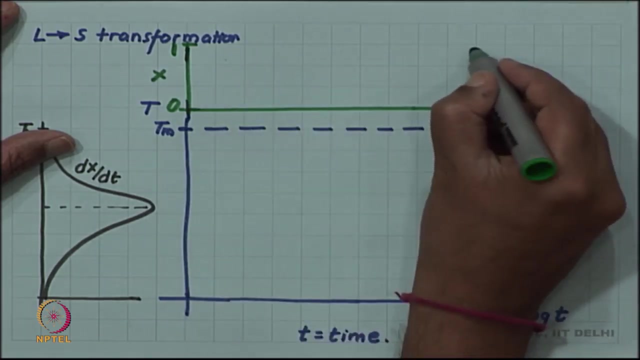 it goes through a maximum at some temperature, where this is the overall transformation rate d x by d t. Also, at any given temperature, we have seen that the transformed fraction x transforms between 0 to 1 as a function of time, and has some sort of s curve. 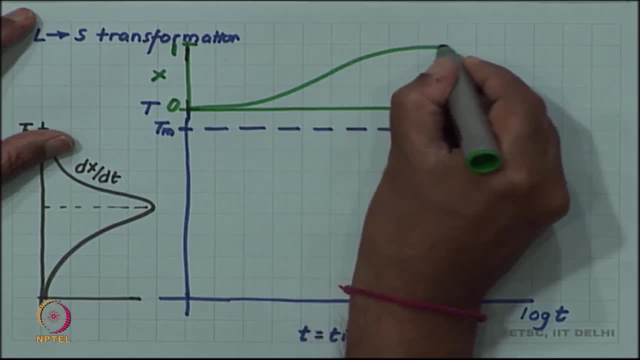 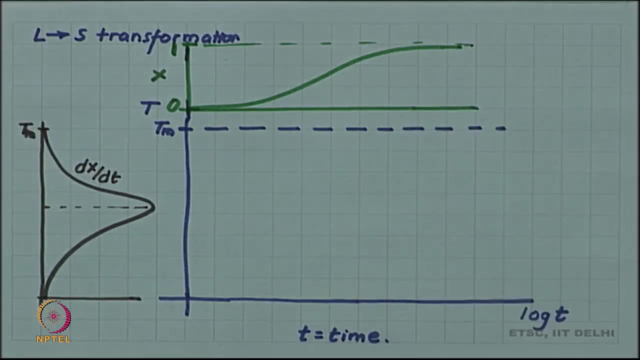 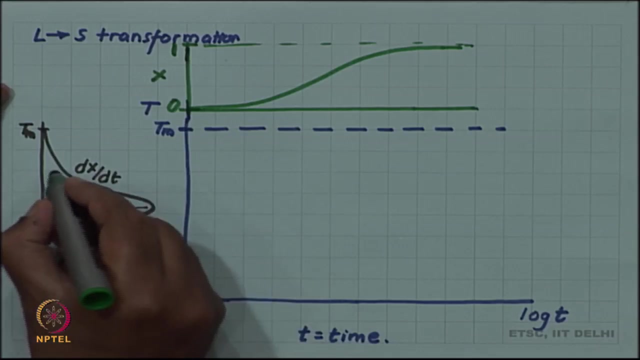 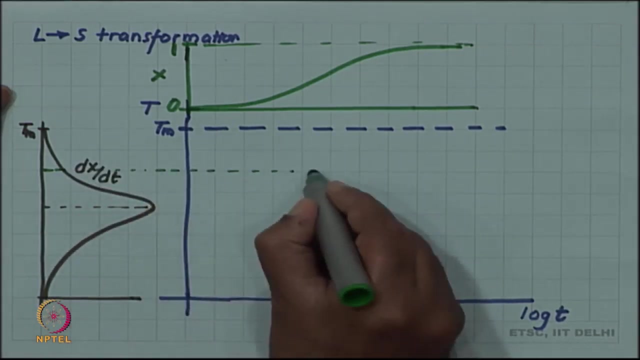 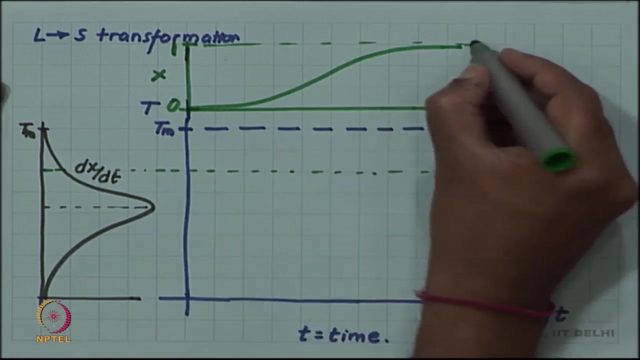 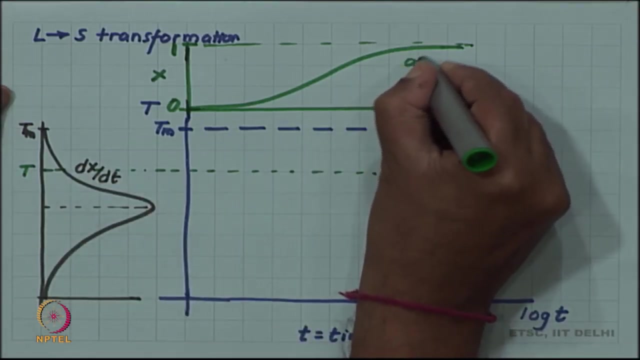 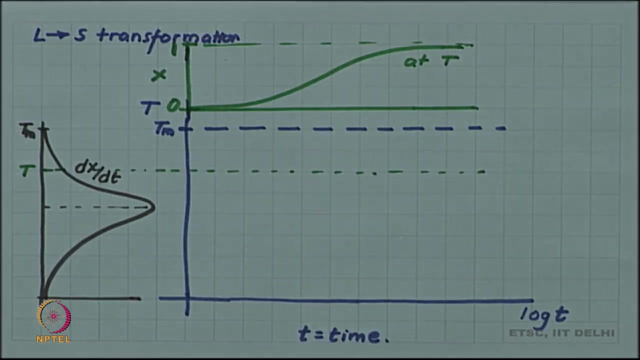 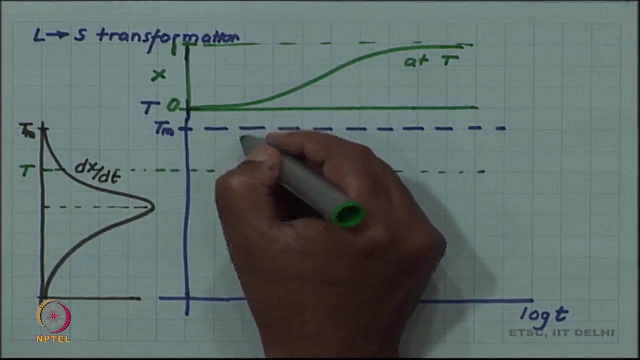 Question. So let us say that we have drawn this s curve at this temperature, So at this temperature. this S curve will obviously change at different temperatures, So at this temperature. what I can do is to plot the time for the start of the curve, the start of the transformation. 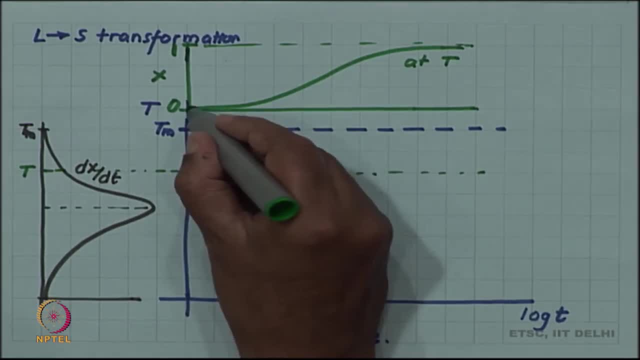 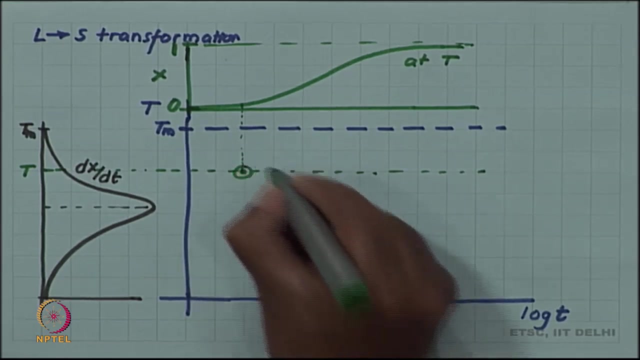 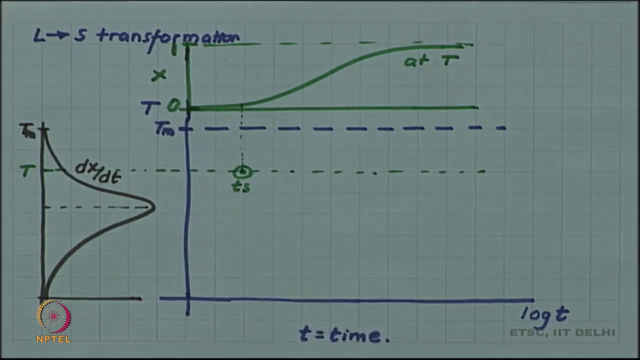 So you can see here, initially the transformation volume fraction transformed was very negligible and will not be detectable. At the point where it reaches some sort of detectable level, that will be our start time. So we mark that as our start time. T: s and after some time the 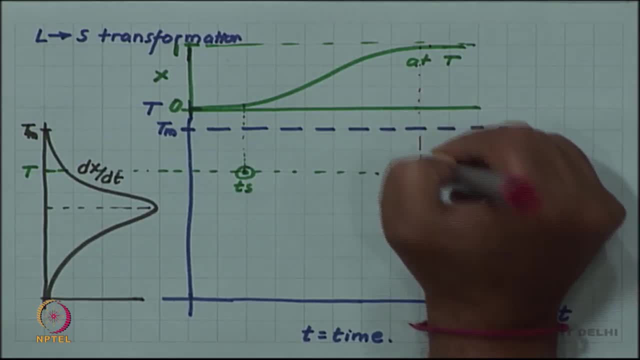 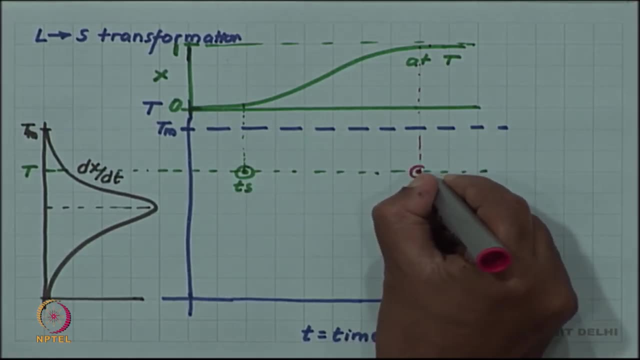 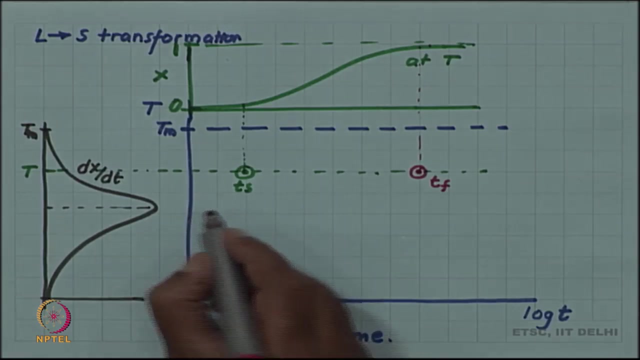 fraction will reach very close to transformed fraction of 1.. So that time we can call as time for finish, And obviously, at the maximum temperature, at the temperature at which you have the maximum rate, both the start time and the finish time will be shorter. The start 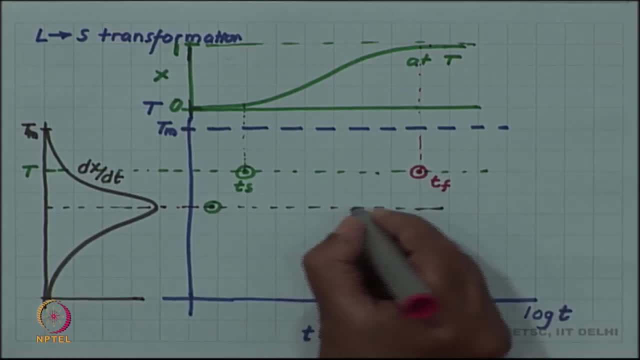 time will be here in the finish time because the transformation rate is fastest, So the transformation will complete in the shortest possible time. it will start in the shortest possible time. It will finish also at a shortest possible time. but if we go lower than this temperature, 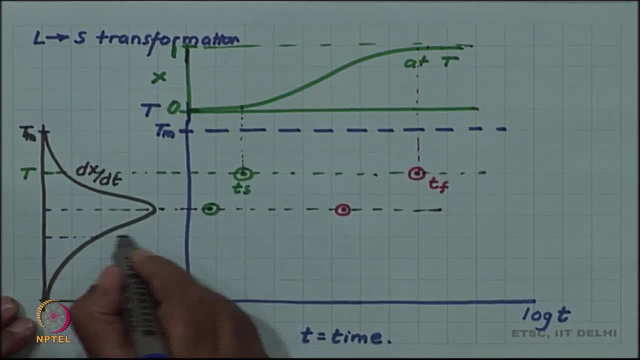 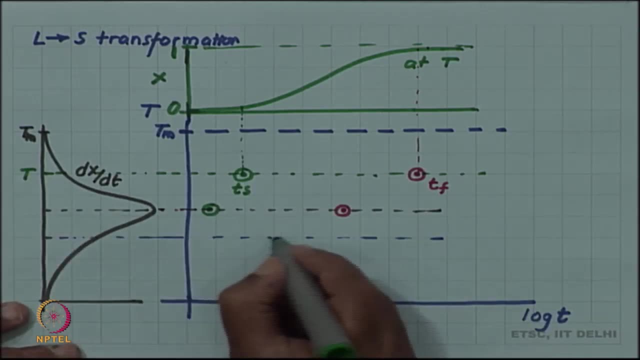 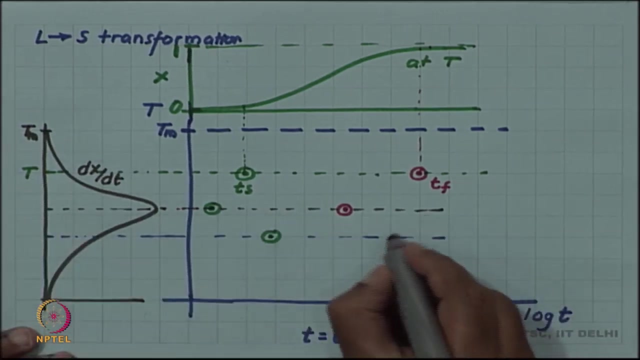 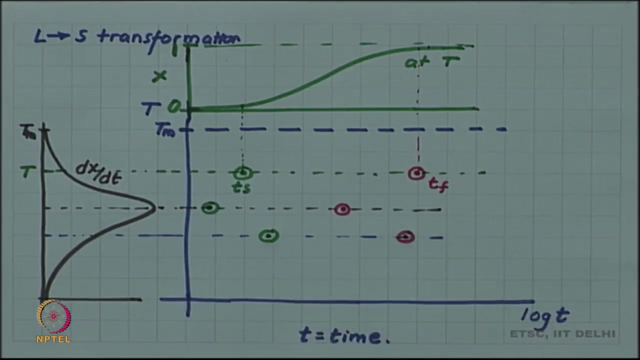 if we lower the temperature further, then the time to start and finish will again start increasing, and if we go to a still lower temperature, So the rate for transformation- this is the transformation rate- is still smaller, So the time to taken to transform will keep increasing. 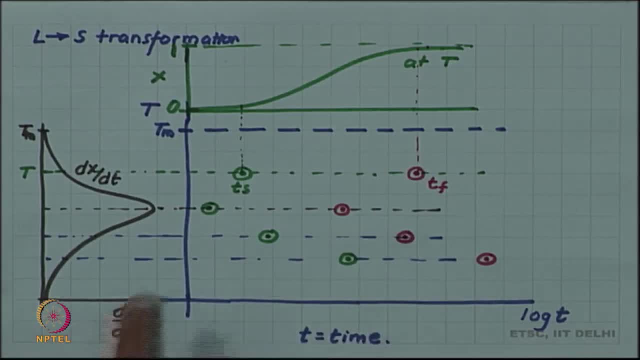 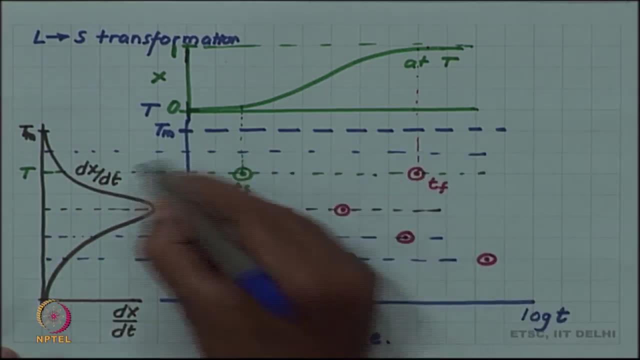 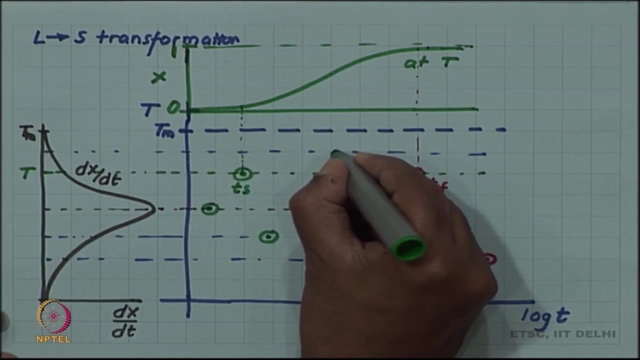 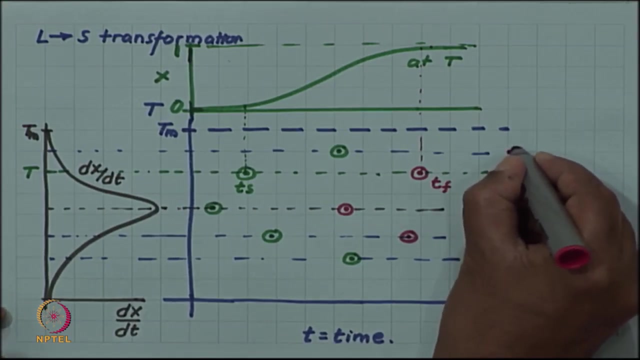 And similarly at high temperature. you can see that as you try to reach closer and closer to the melting temperature, the reaction is becoming slower and slower. the transformation rate is becoming slower and slower, So you will take more and more time to start and finish the transformation. So if we now in this diagram connect all the 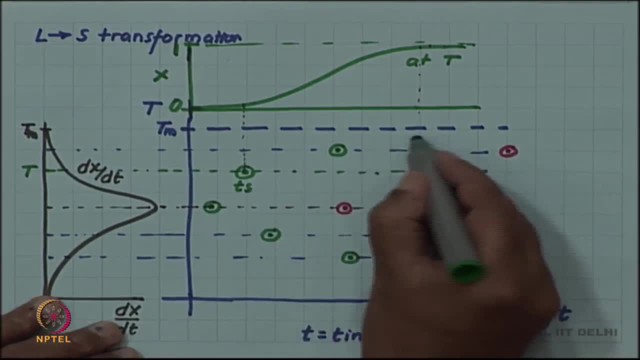 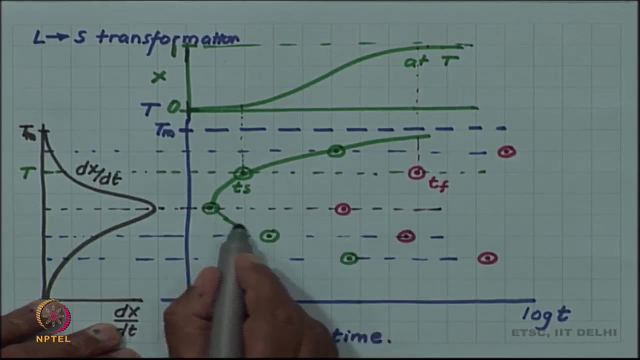 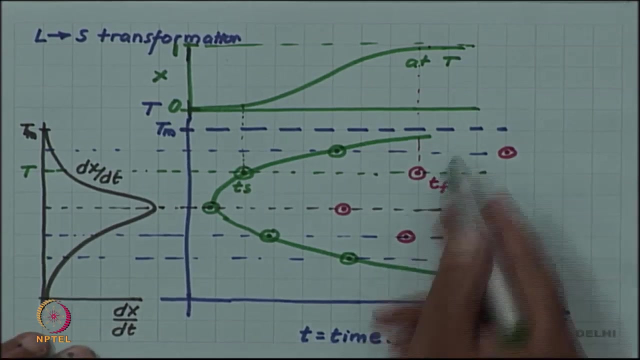 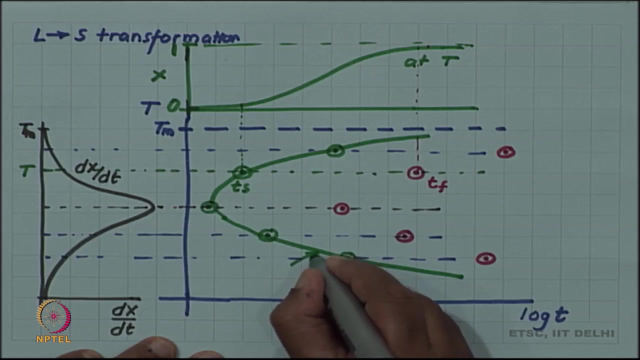 start times. So these green points are a start time. by a single curve We get a C curve. you can see the shape of the C curve. this is a C curve and this is the start curve. so I label this as time, fot, start or t f. 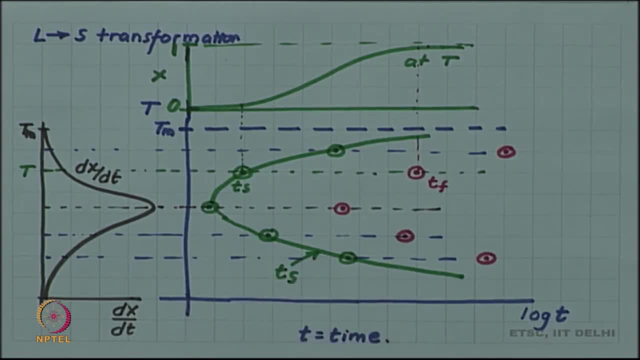 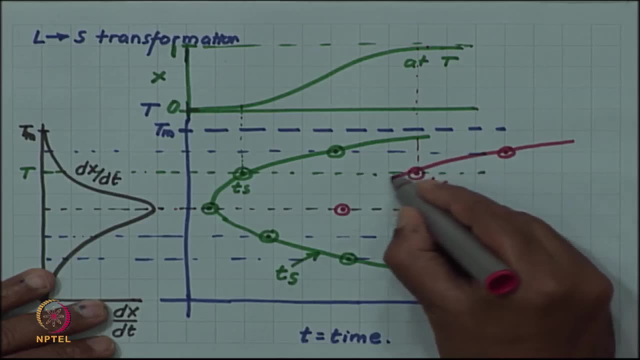 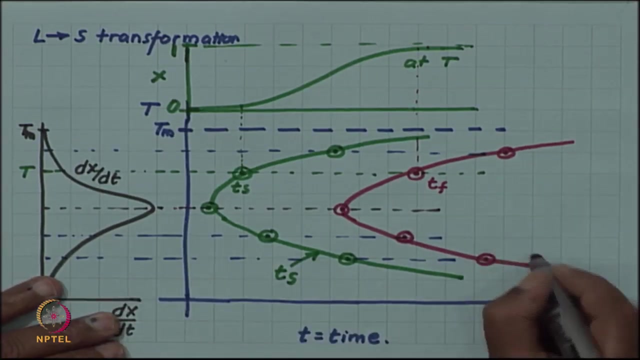 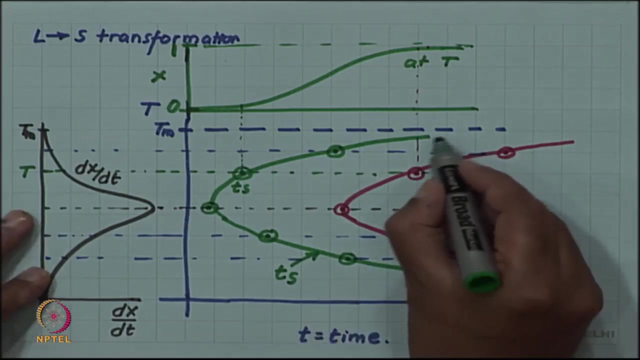 s. And if I connect all the these red dots which were representing the finish time, then I get another curve and this is the time for finish. So both these are called C curves and both will approach at the higher temperature side, both will approach asymptotically the 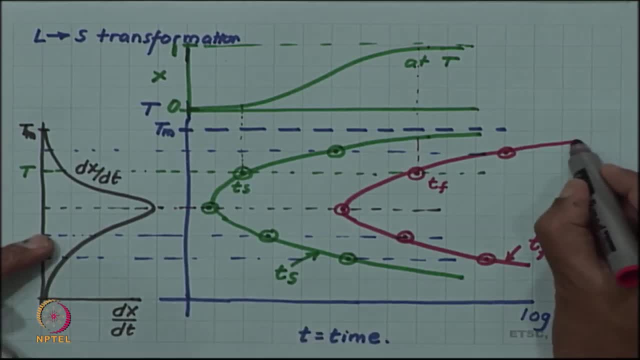 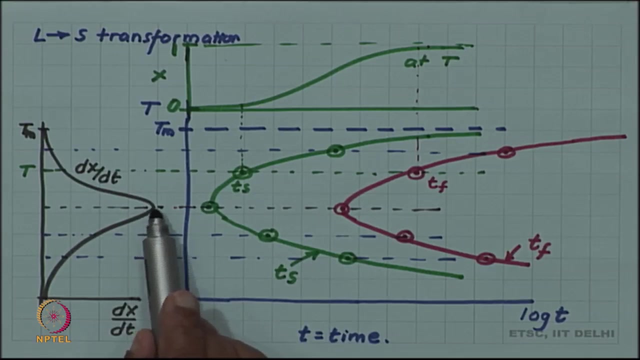 melting point. they cannot cross the melting point because there is no transformation above the melting point, but they will reach asymptotically the melting point And at a point where, at the temperature at which the maximum transformation rate was there, they will show a minimum time and that is usually called in the known as C curve. 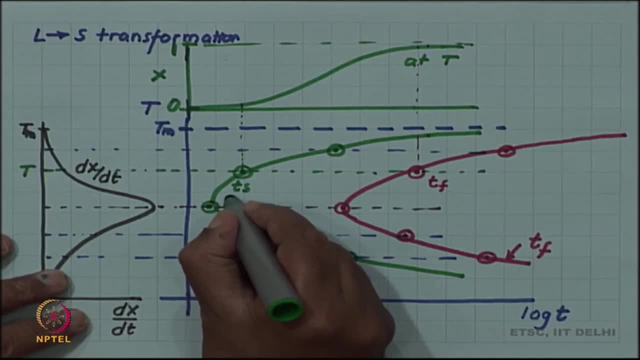 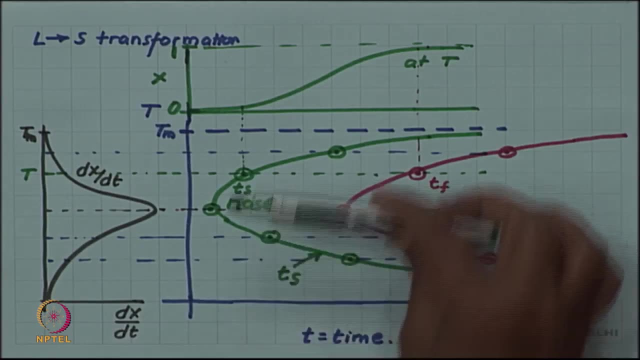 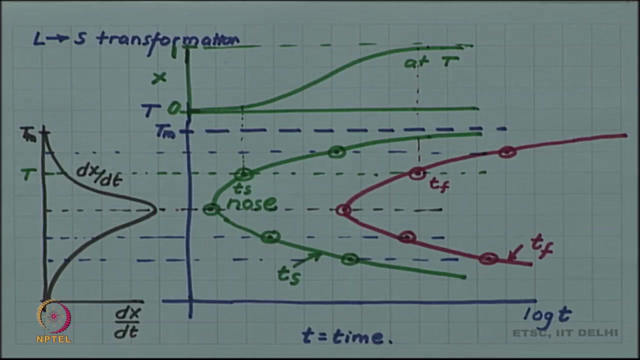 nose of the curve. So this is the nose, and above and below the nose you have longer time than corresponding to the nose. Now from this diagram we can interpret how the transformation is happening. So we are drawing t t t diagram. t t, t, t, t t t. 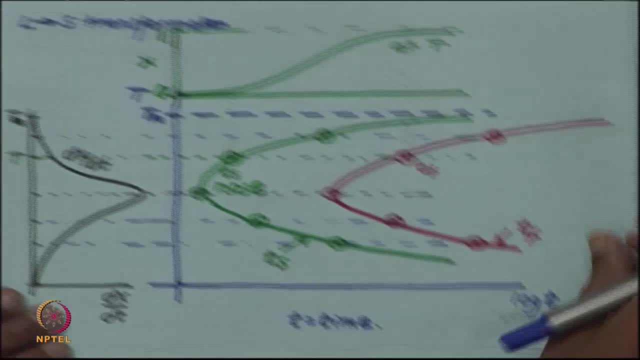 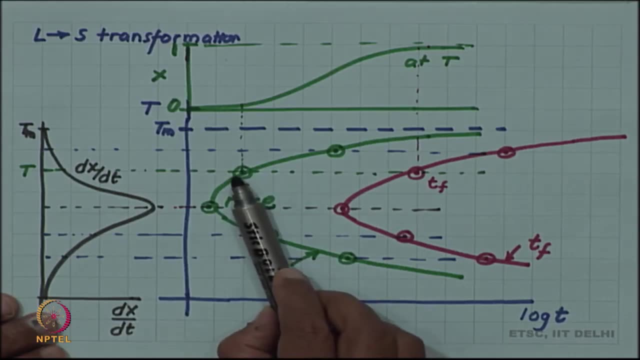 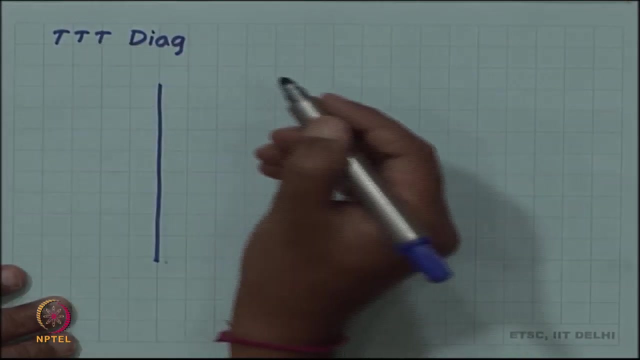 time temperature transformation diagram. you can see it has a time axis, it has a temperature axis and it is representing the transformation: start time for the transformation and finish time for the transformation in the diagram. So that is why we call it with 3 t time temperature. 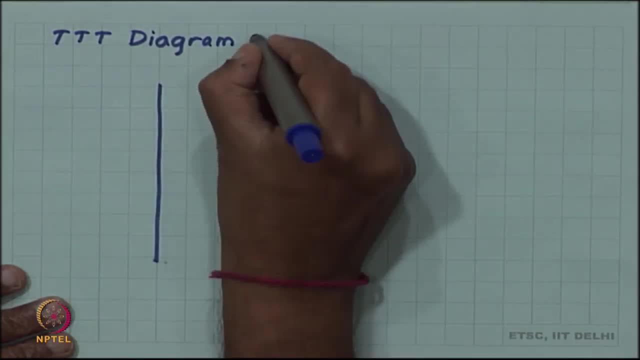 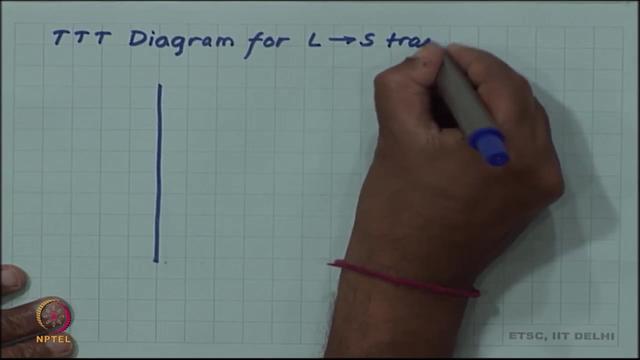 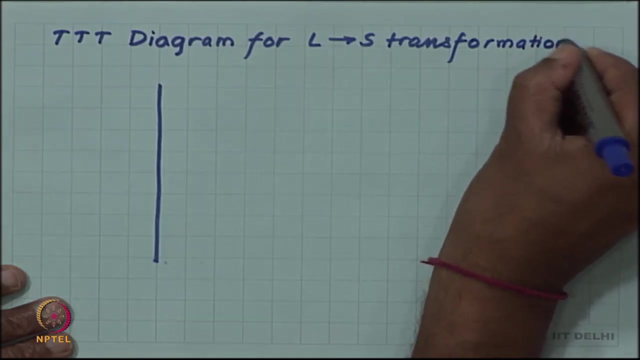 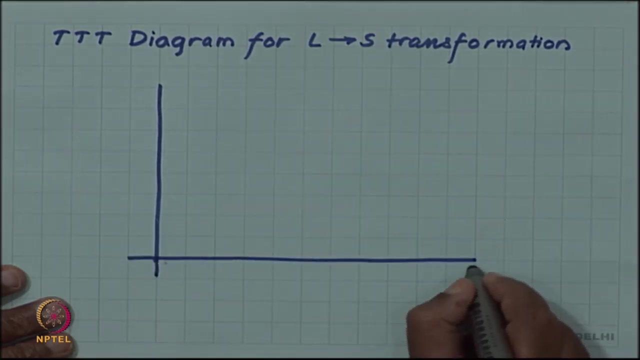 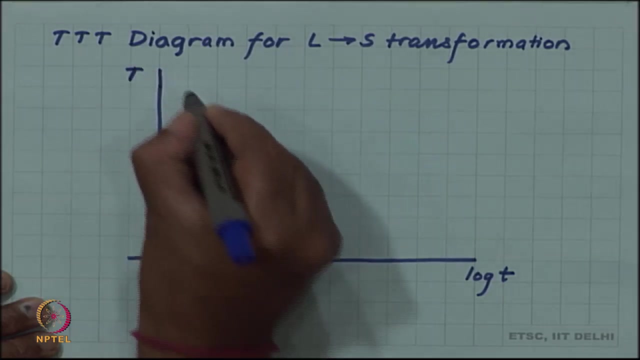 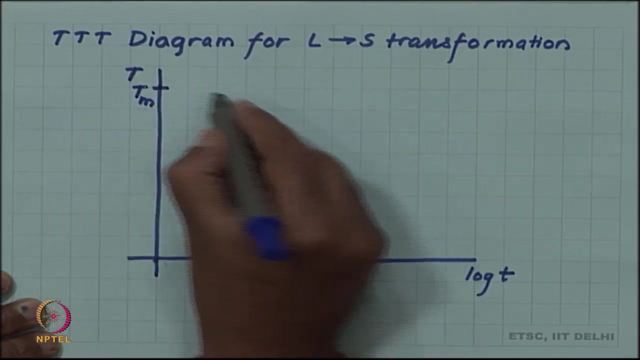 transformation diagram. So time temperature transformation diagram for liquid to solid transformation. These are the two axis. you have the time axis in logarithmic scale. you have the temperature axis. in temperature axis the critical temperature is the melting point Above the temperature. 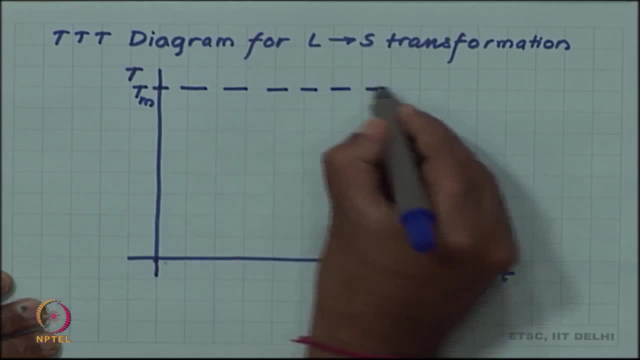 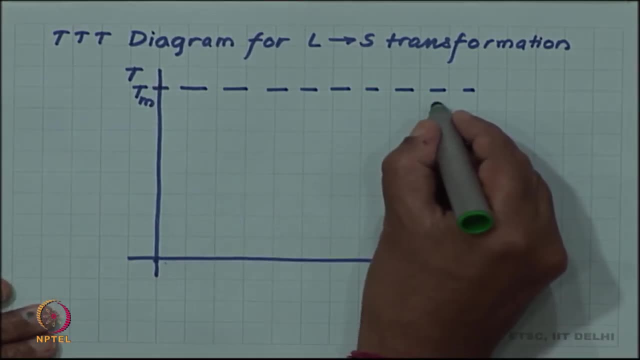 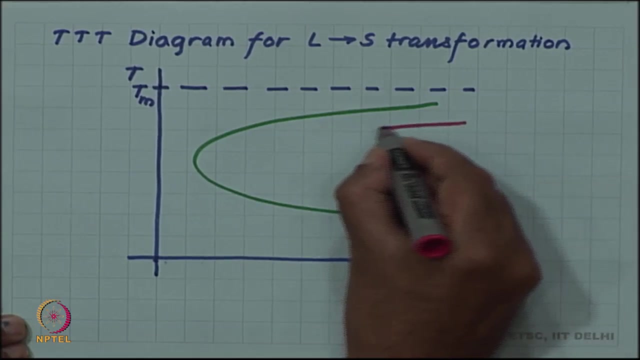 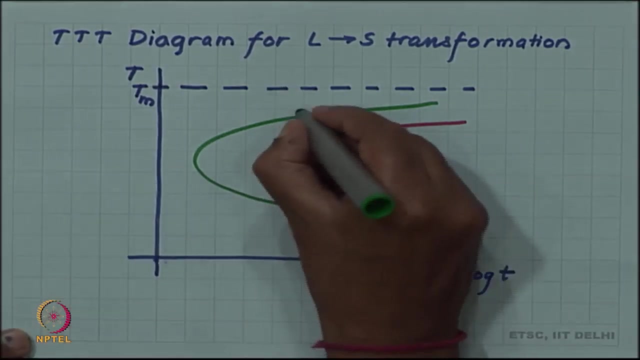 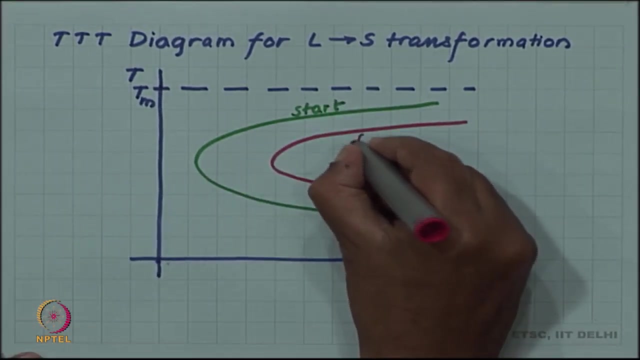 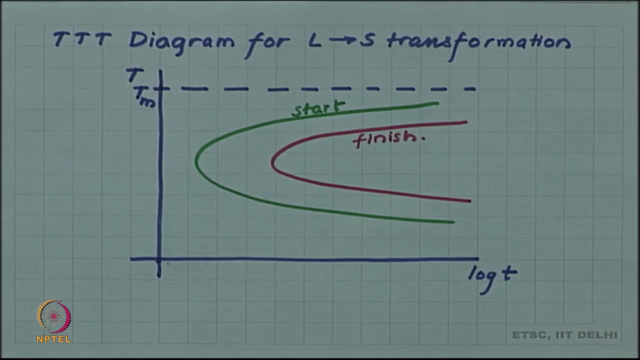 is the melting point, above which nothing happens. and then we saw that there were two C curves, one for the start time and one for the finish time. So this is the start time, the start time, the end time and this is finish. 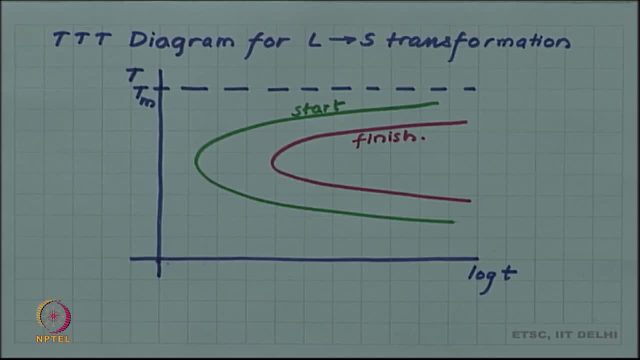 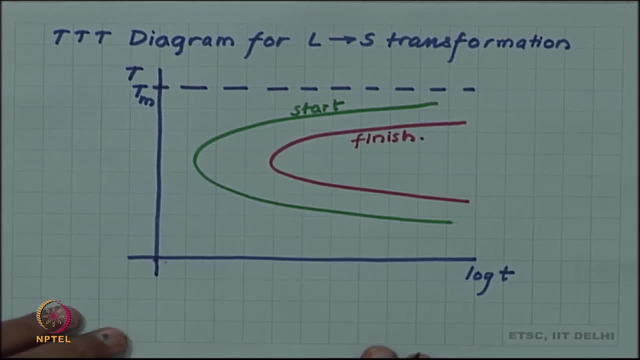 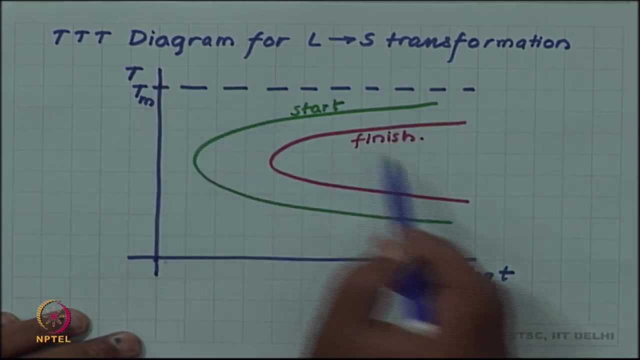 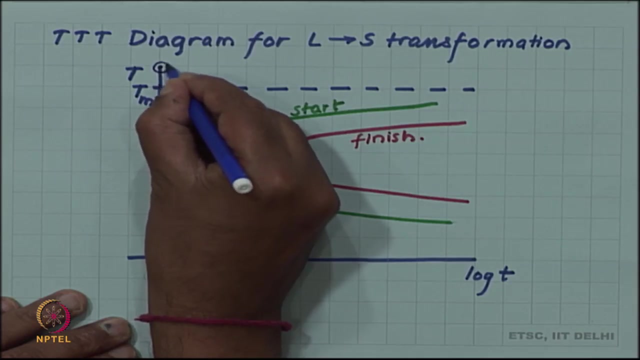 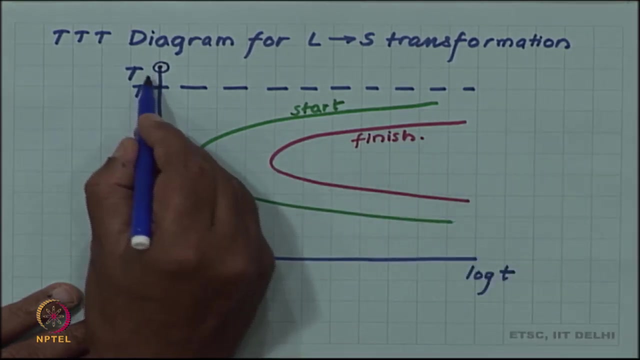 Now we can superimpose on these curves the cooling curve for the alloy, So cooling curve for the liquid. So as the liquid is cooling, let us say start with the start time, then liquid at a temperature higher than the freezing temperature, T, m, and then from there we gradually 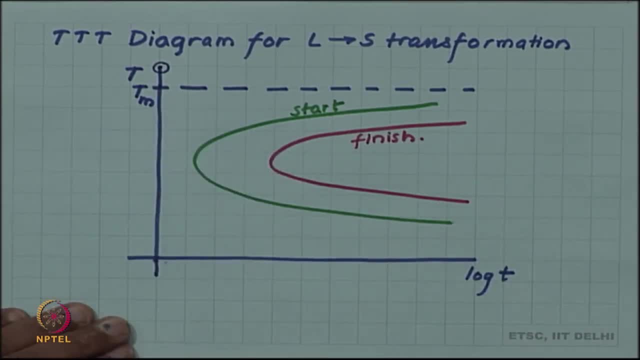 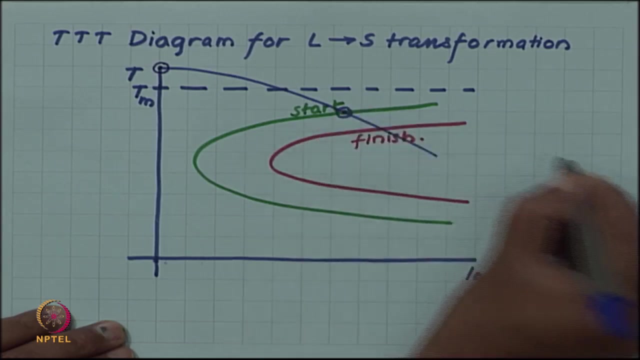 cool this. So you can see that if I am cooling it, at some point it will hit the start curve and the crystallization will begin, and at some point it will cross the finish curve and the crystallization will finish. Although the way we had drawn this diagram was for 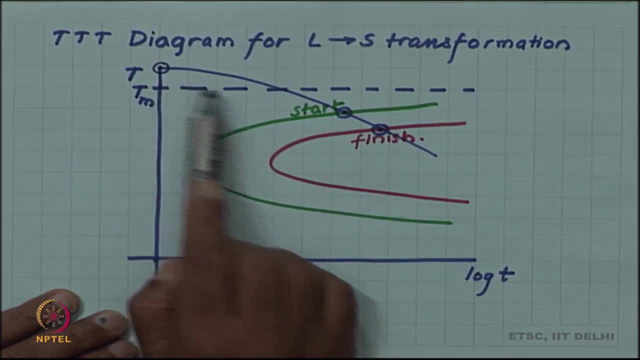 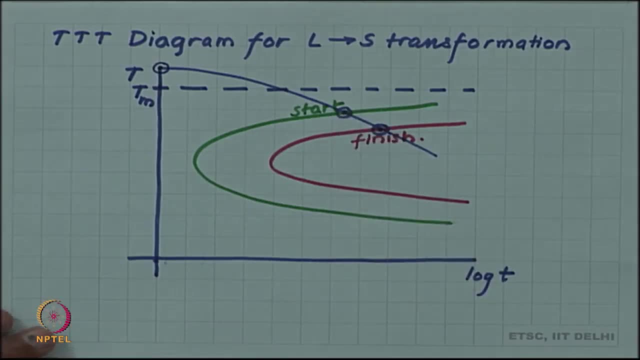 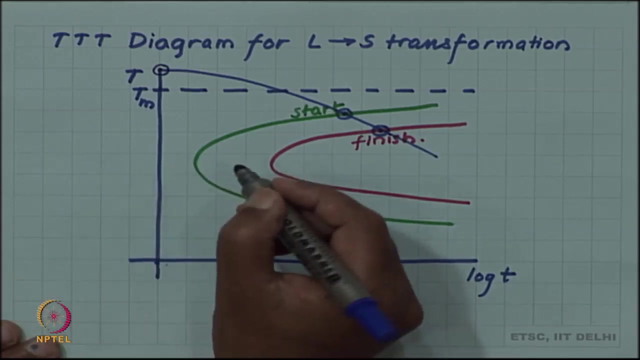 isothermal transformation. So it will not be directly applicable for such cooling curves, but approximately we can take these temperature as the temperature for start and finish for this continuous cooling diagram also. So before you can see, before the start curve, So let us first label the phases. So before 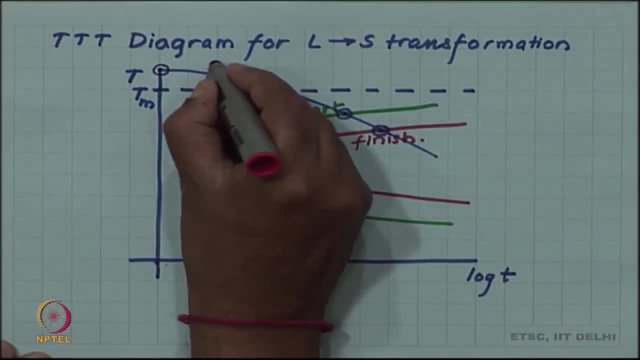 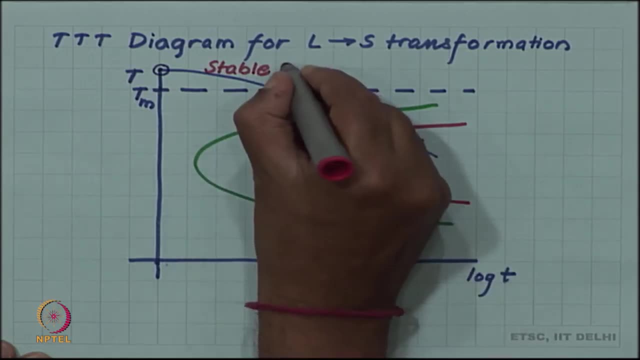 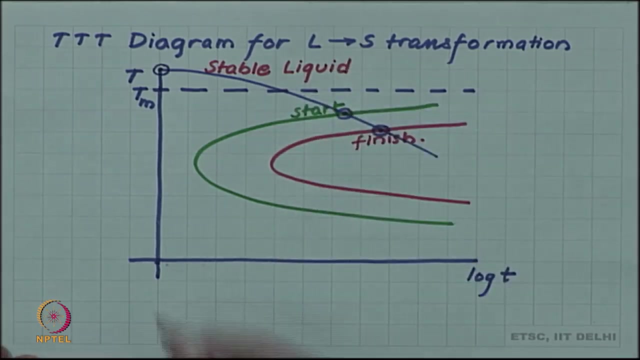 the start, above the melting point you have liquid and that is a stable liquid. that is a happy liquid it is. it does not want to transform. So we have a stable liquid Below the melting point. So the liquid should transform, but before the green curve the transformation has not. 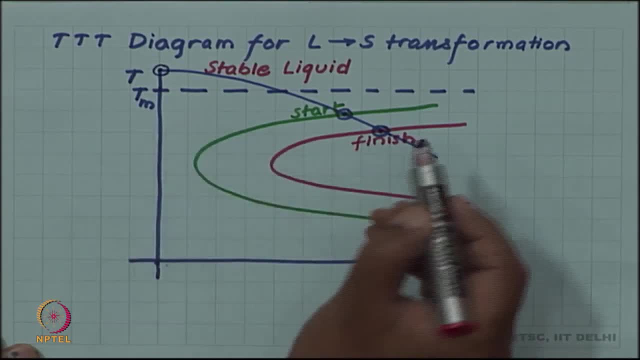 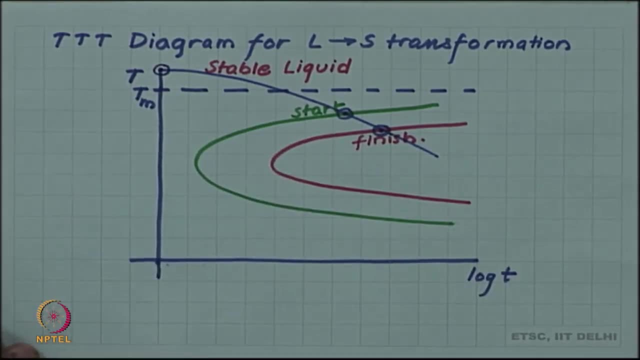 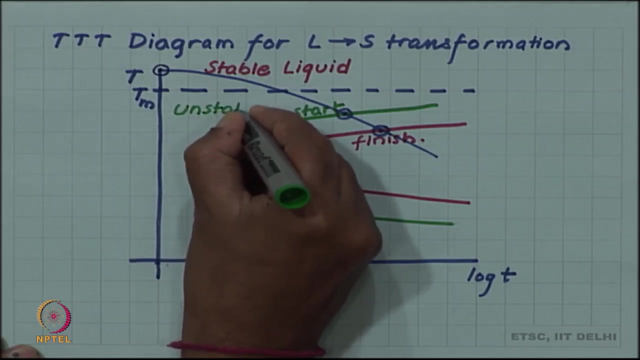 started. So you have a liquid which wants to transform but has not yet transformed, So that is an unstable liquid. So below this, here you have unstable liquid, or also called undercooled liquid. So below this, here you have unstable liquid, or also called: 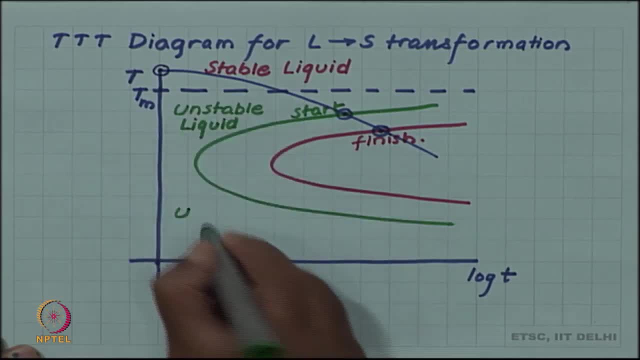 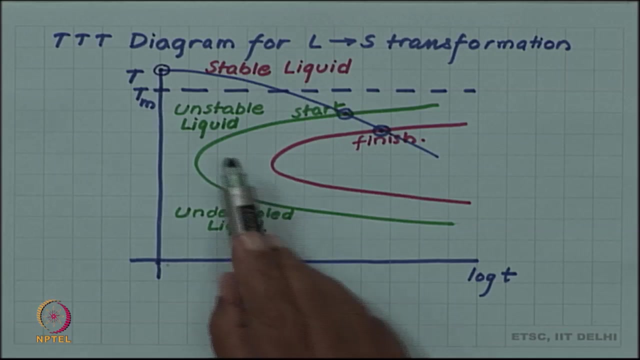 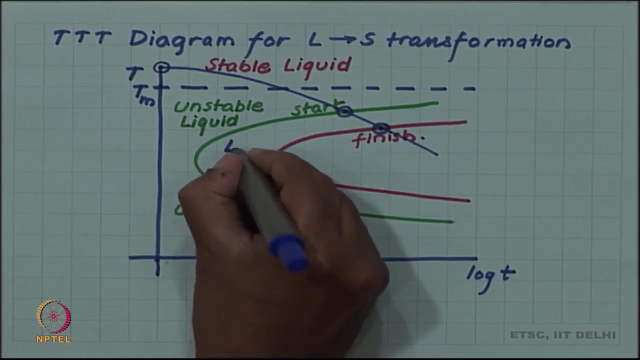 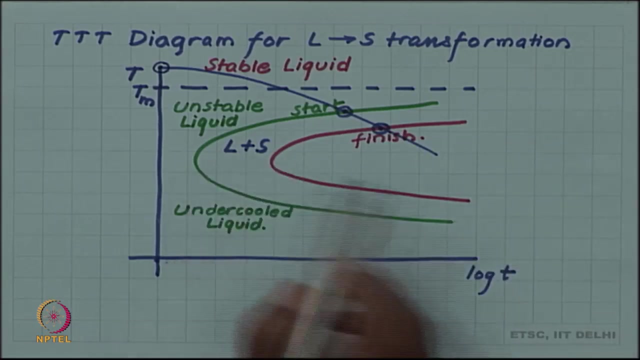 undercooled liquid, because this is a liquid below the melting point, So we can call it undercooled liquid. Then, beyond green line, the transformation has started. So you have liquid as well as solid. So liquid has transformed into solid, but some liquid is remaining Beyond the red curve. 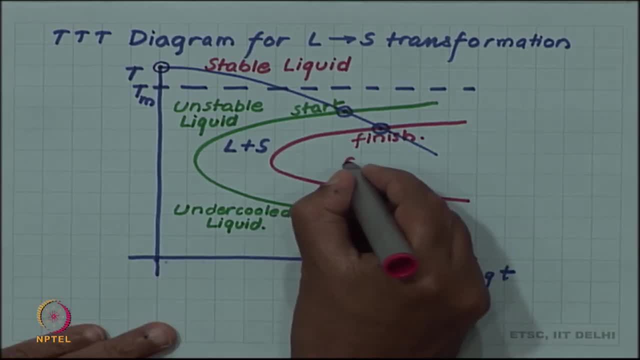 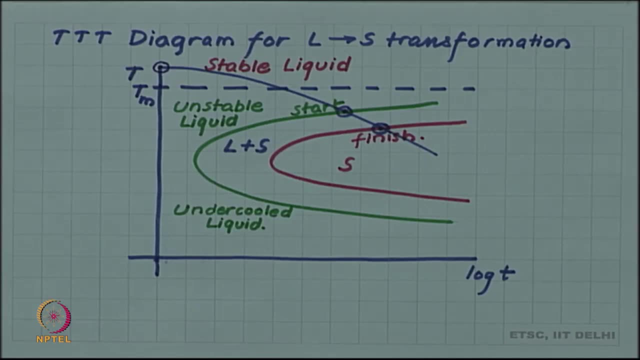 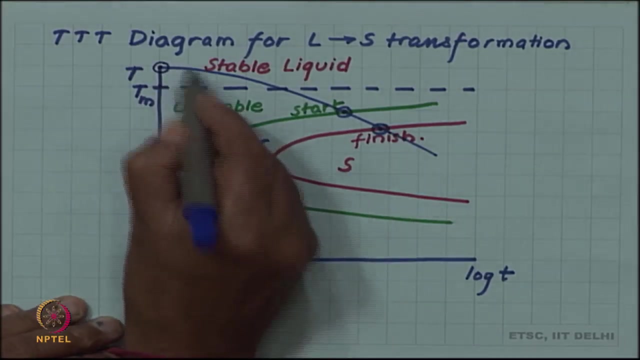 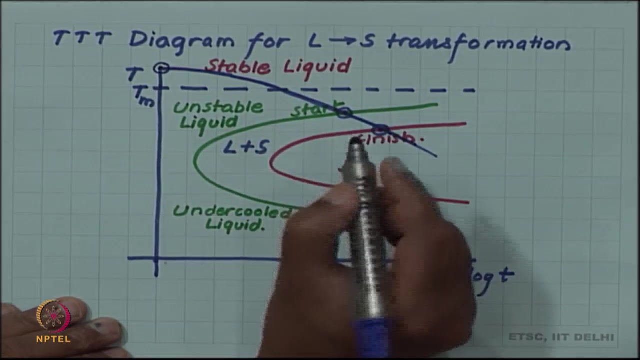 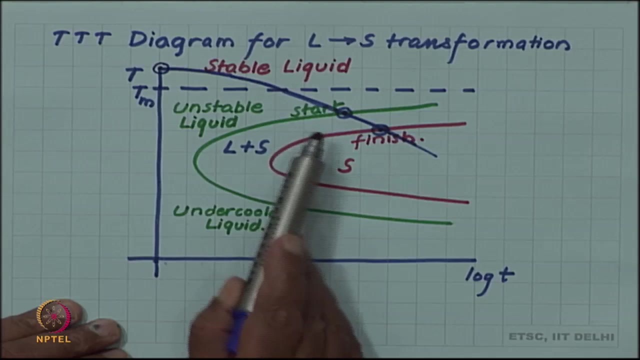 the transformation has completed, So you have only solid. So if we now follow this blue line, if we now follow this blue line, So the transformation begins here and then completes here. So finally, from stable liquid it goes into undercooled liquid and then starts transforming into solid and completes the 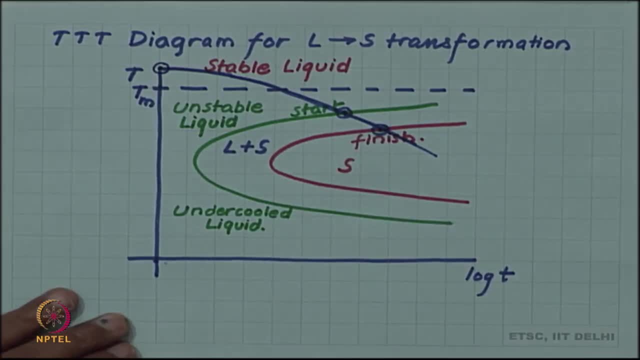 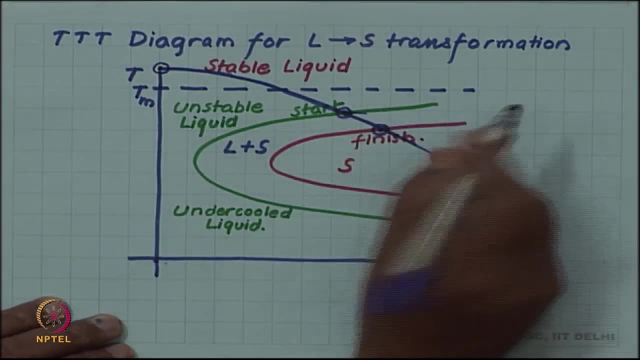 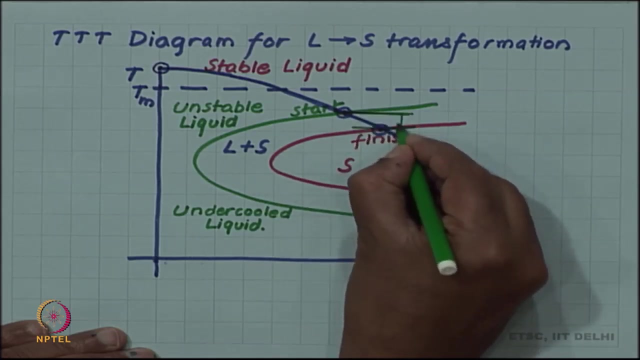 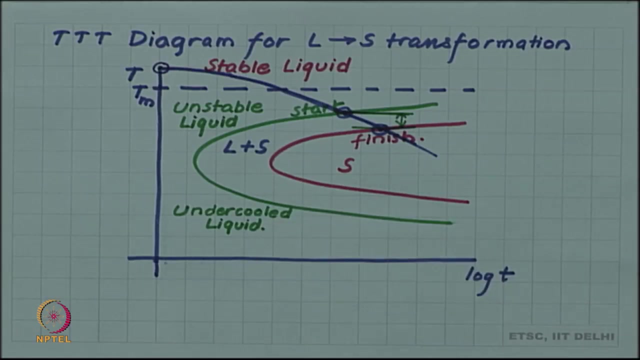 solidification, The temperature range over which this transformation happens can be seen. This menu can be seen as this range, And let me label this, this line, as a slow cooling, In comparison with another line which I am going to draw now. this is another total mass that we can put into this. 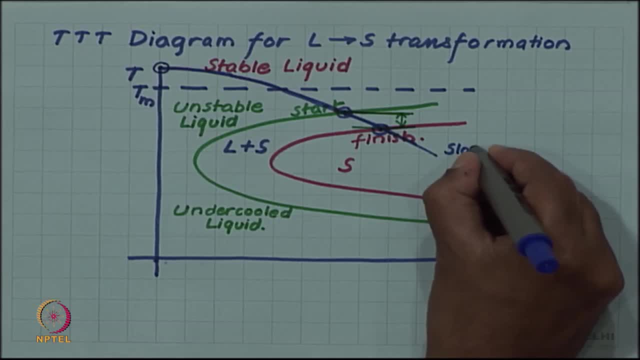 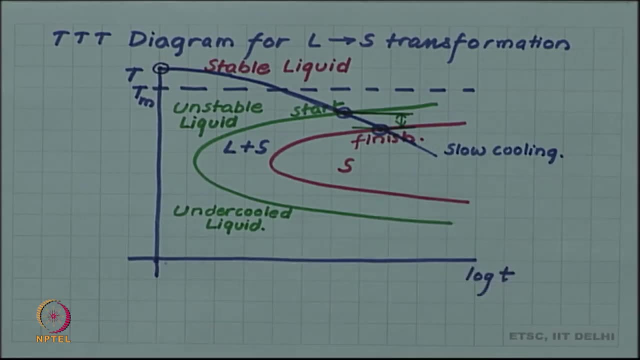 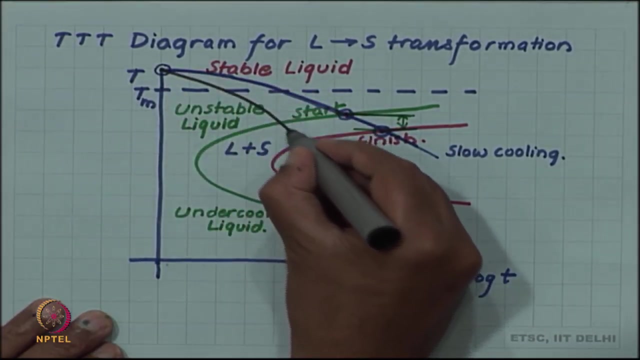 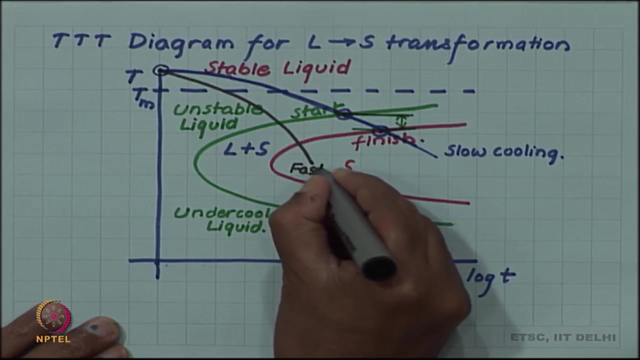 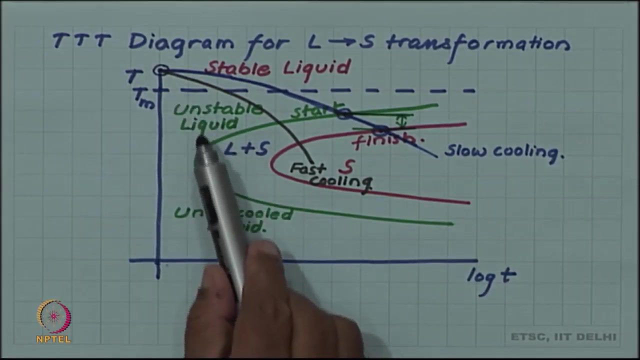 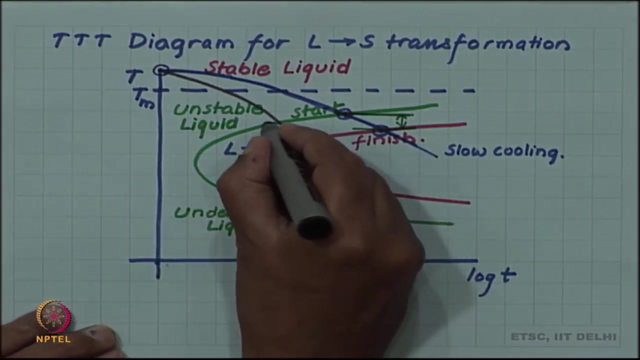 fluid In comparison with another line which I am going to draw now, which will represent a faster cooling, because you can see that the temperature is now falling much more rapidly compared to this blue line And if you now compare the temperature range over which this transformation is happening, 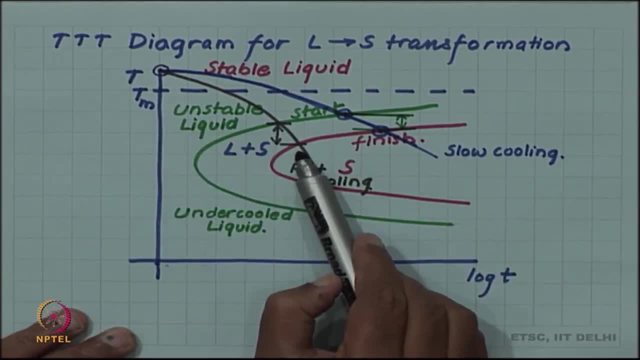 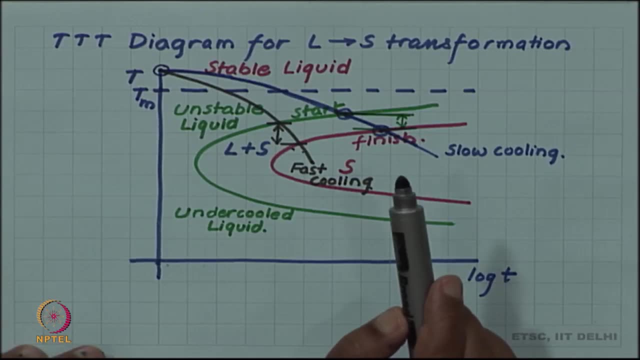 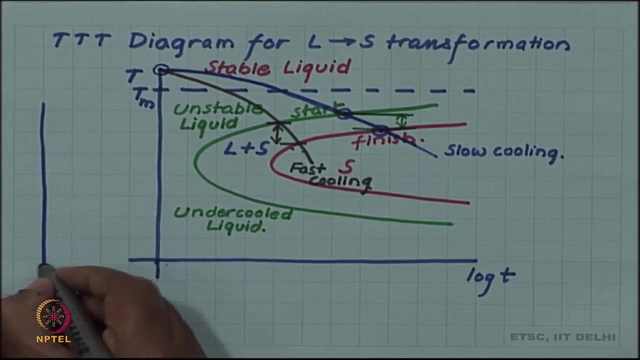 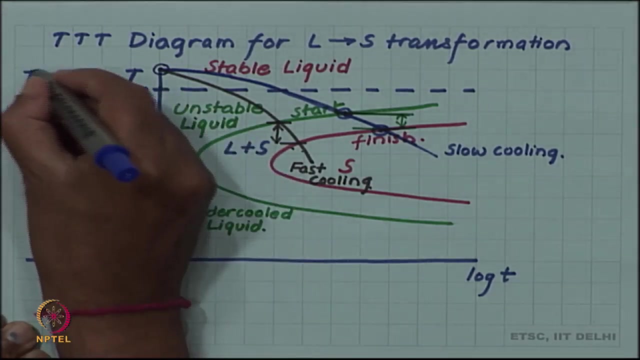 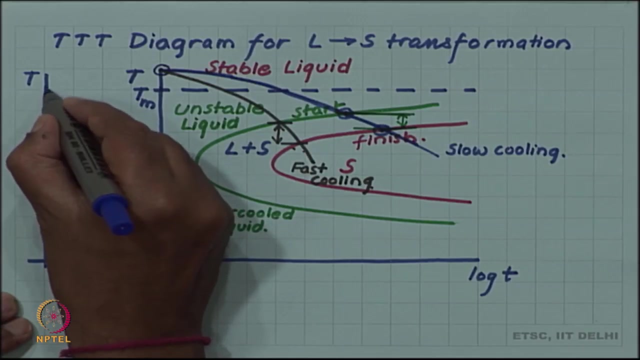 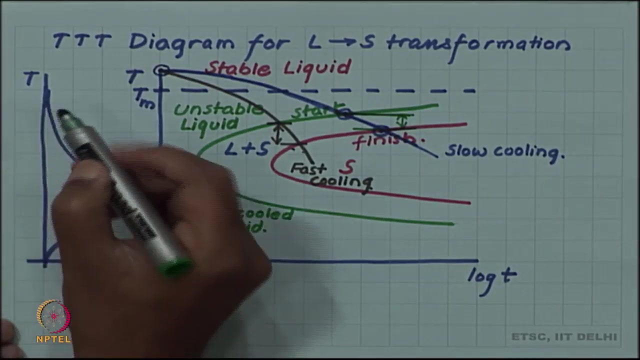 is this? So, on faster cooling, The temperature range over which the transformation happens is lower than in slower cooling. This you can then relate with your nucleation and growth rates. So remember that there was a nucleation rate maximum And there was a growth rate maximum. 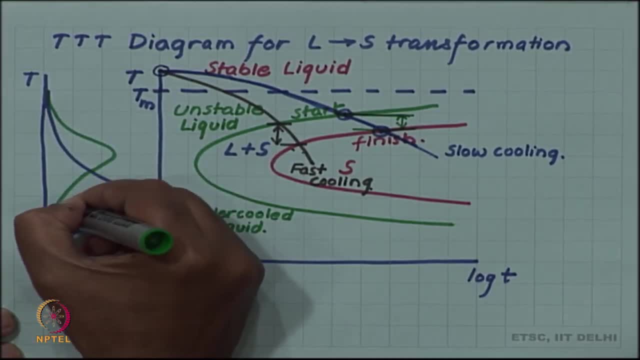 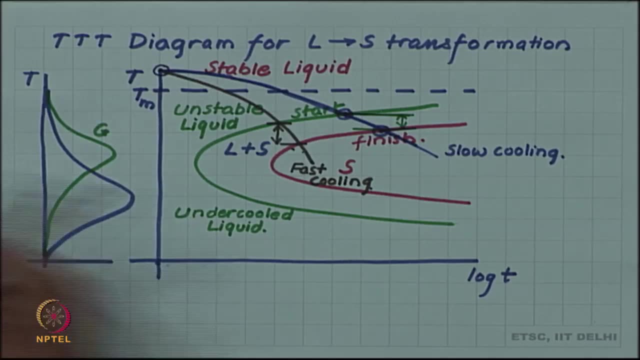 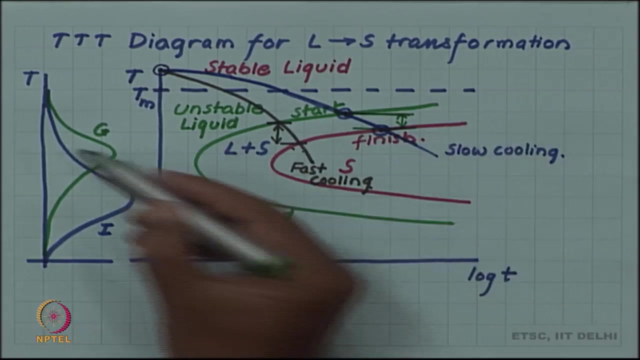 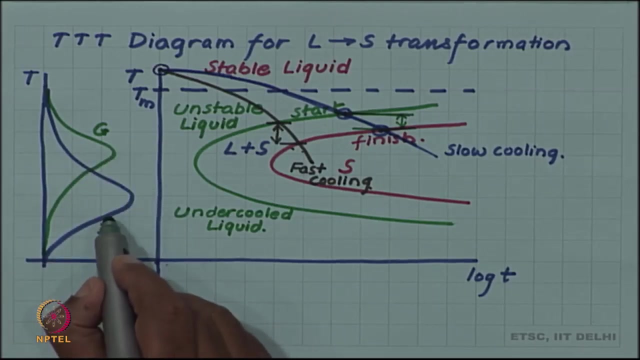 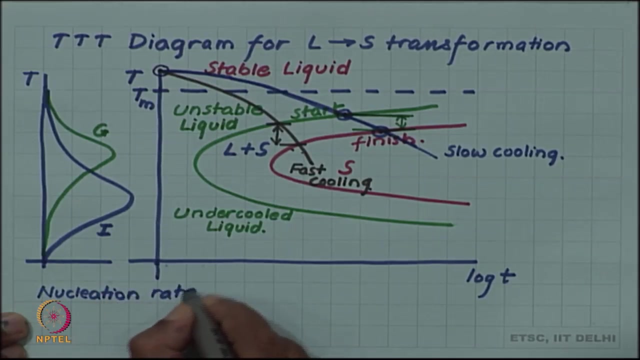 So on the higher temperature side, growth rate is dominant compared to the nucleation rate. On the lower temperature side, the nucleation rate is dominant compared to the growth rate. Let us note that Nucleation rate is dominant at Ok. 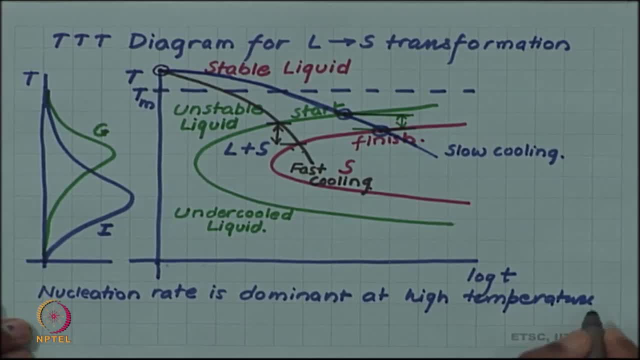 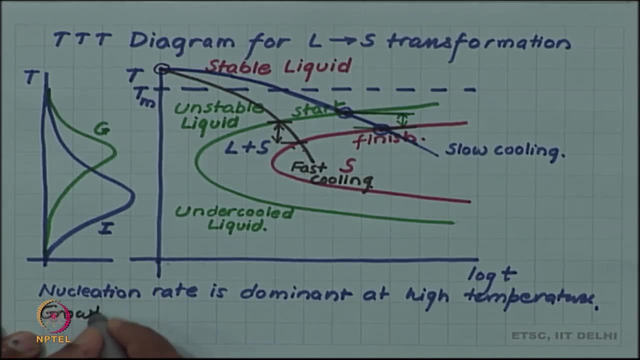 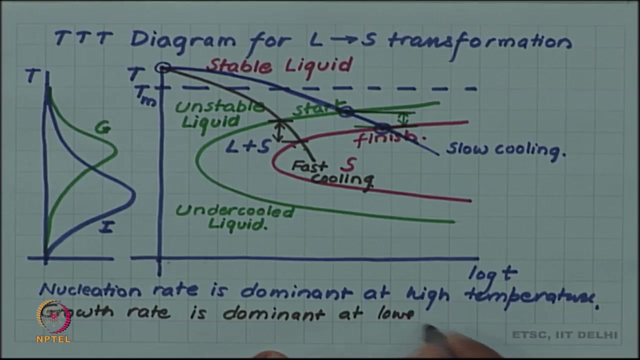 high temperature growth rate is dominant. sorry, I just made a mistake. nucleation rate is dominant at low temperature. you can see from the diagram here: growth rate is dominant at high temperature. Now you can imagine what is happening in your. 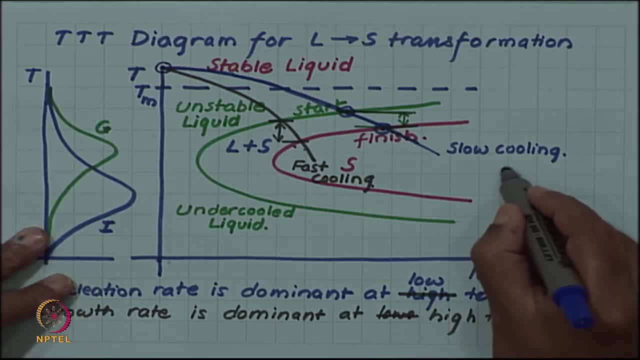 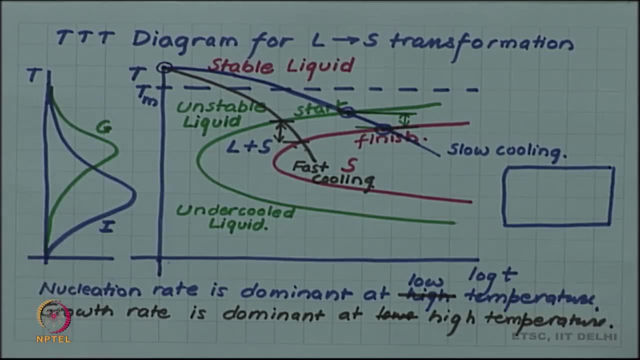 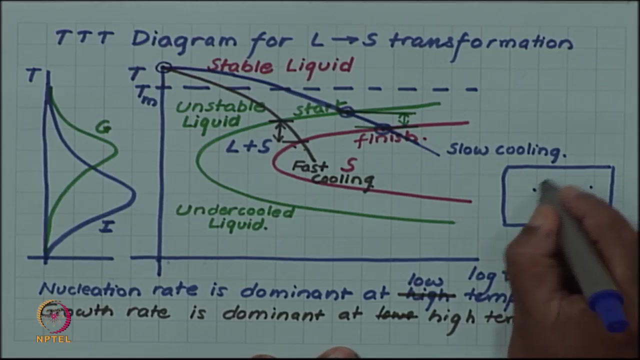 liquid. So if you have a liquid And in slow cooling the transformation temperature was higher so the growth rate is higher and growth rate is more dominant than the nucleation rate, which means few nuclei will form but they will grow very fast. So few nuclei form and they grow very rapidly, So you will end. 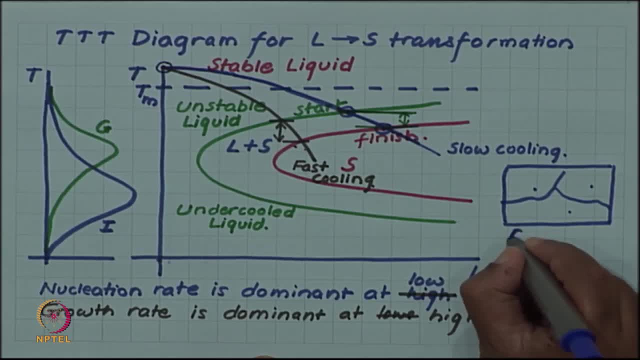 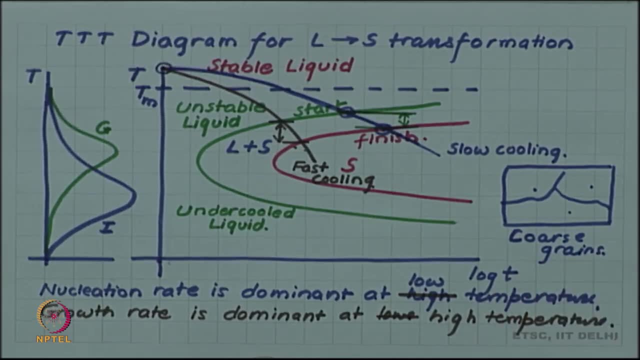 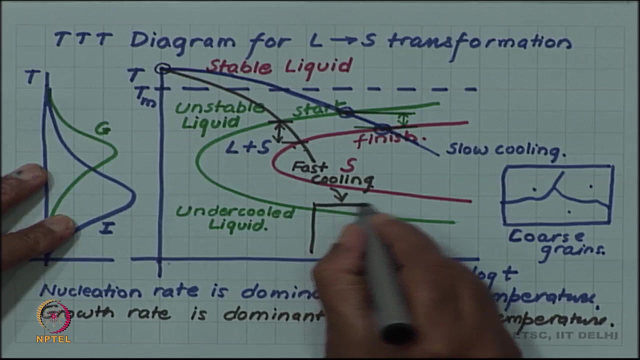 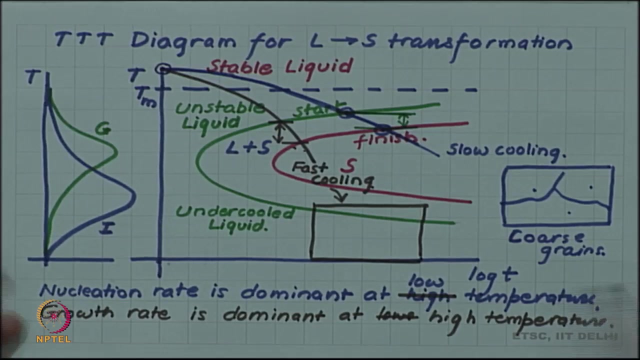 up with large grains or coarse grains, Whereas imagine what will happen in the faster cooling. Now, in the faster cooling the transformation temperature is lower. On the lower side nucleation rate is more dominant than the growth rate, So faster nucleation gives you. 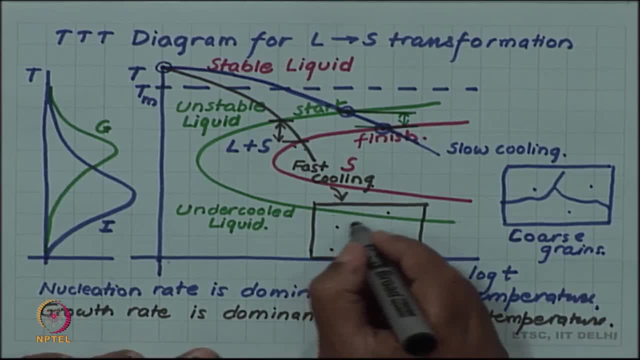 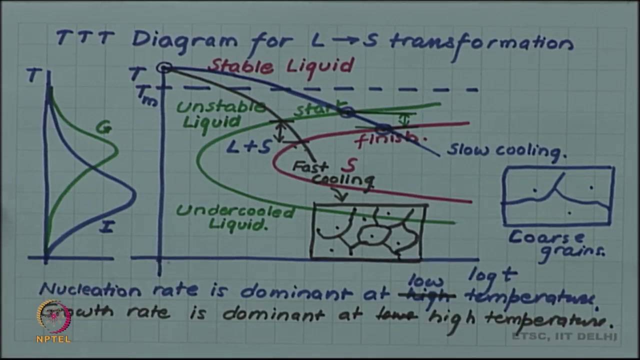 many nucleation center and the growth rate is slow, So they grow at a slower rate, So that provides even more time for further nucleation events to happen. So in the end you will end up with many grains, Because each nucleation event leads to, in the final structure, one grain. So if the 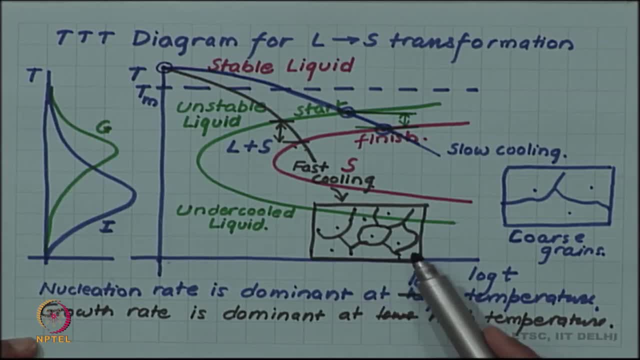 nucleation rate is high, you will end up with more grains And since the total volume of the transforming material is the same, you will have a smaller grain size. So we have finer grains. So this is the normal observation in a cooling of a liquid, that if you have a 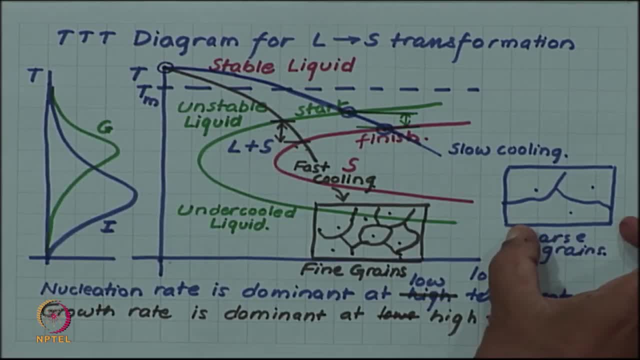 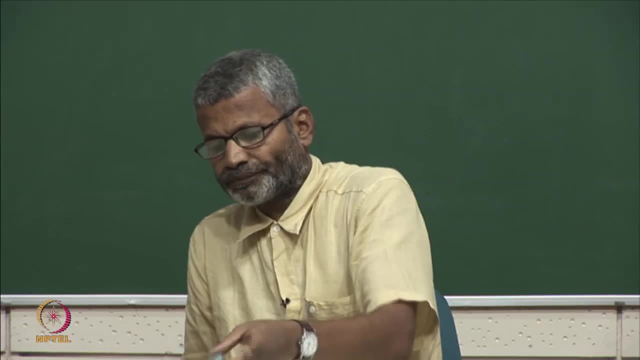 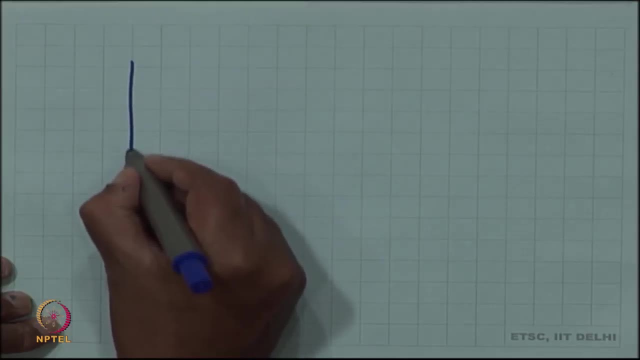 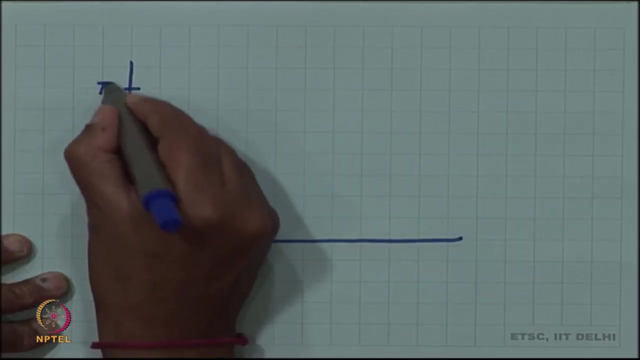 coarse grain. cool it slowly, then you have coarse grain. If you cool faster, then you have fine grains. Now we will compare this with one more interesting case. Now let us have our start: C curve. Now, when it is C curve, it will be E C We would have. 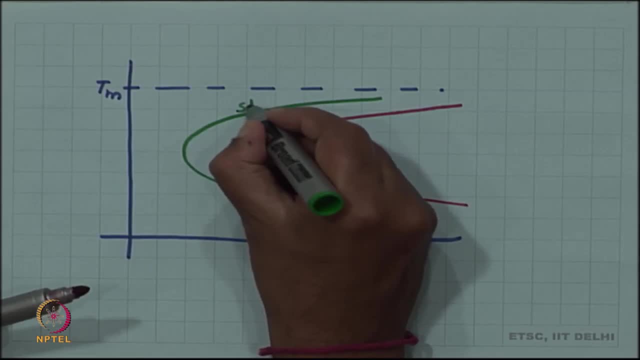 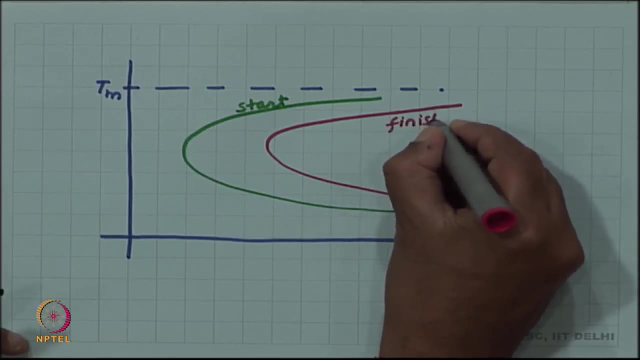 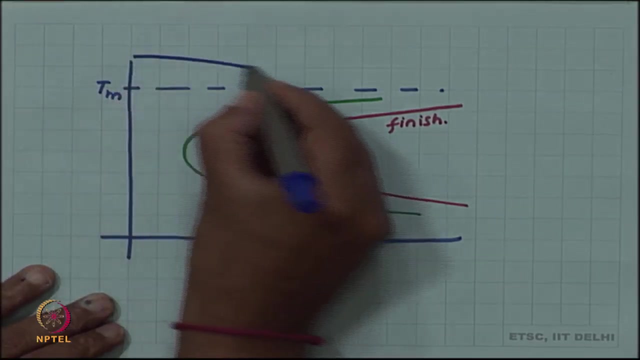 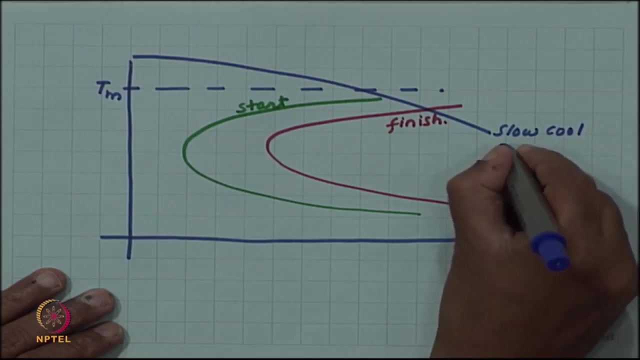 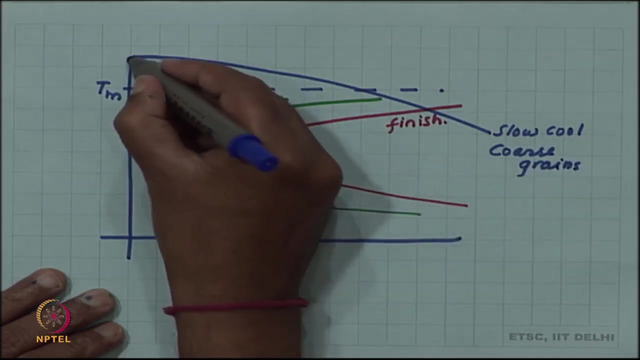 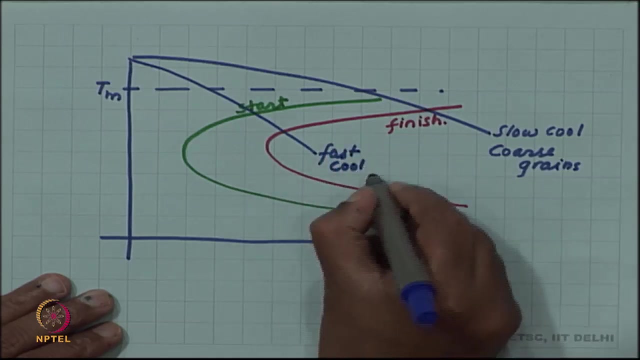 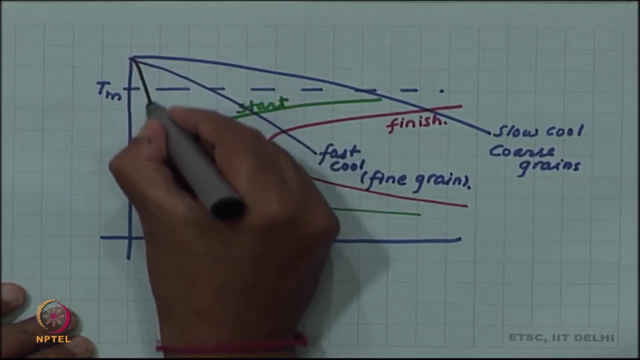 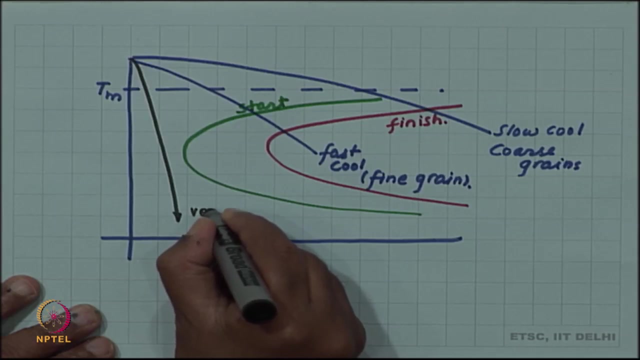 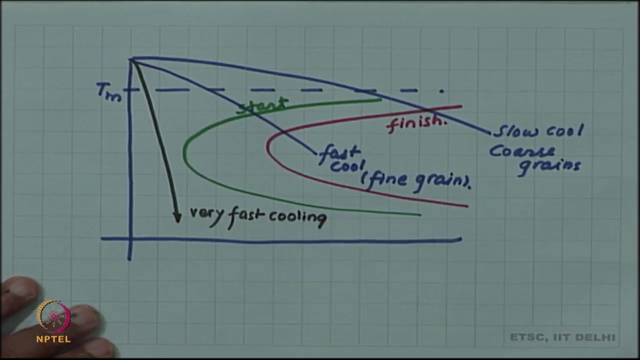 So we saw that a slow cooling gave us coarse green And a faster cooling gave us fine green. But what will happen to a liquid which is cooled this fast? Okay, So very fast cooling, let us call this so here. the cooling is so fast, sometimes this: 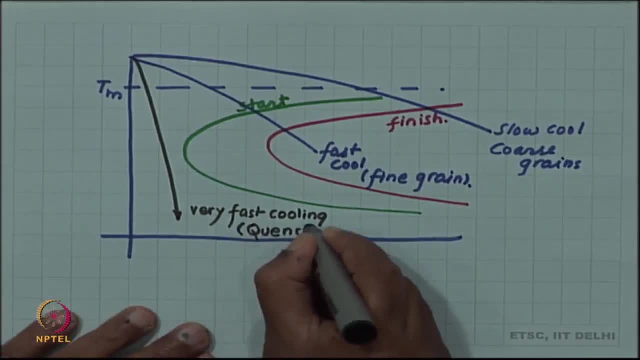 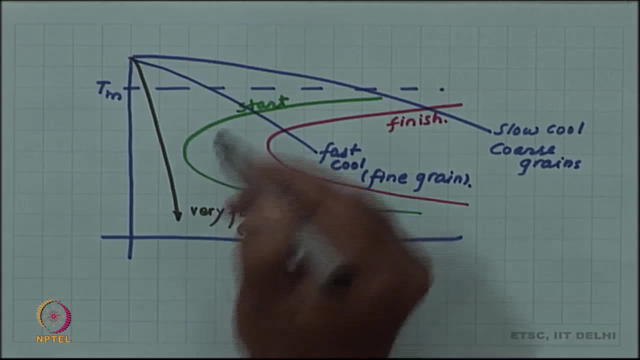 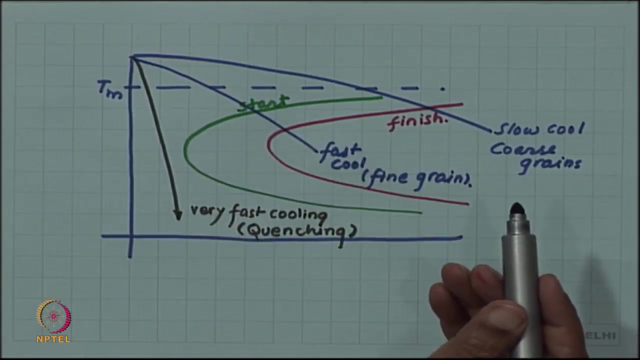 is what is called quenching. so if you cool something very fast, you are quenching the material. So if the liquid is quenched so fast that it even misses the nose of the start curve, so the solidification is never starting in this. 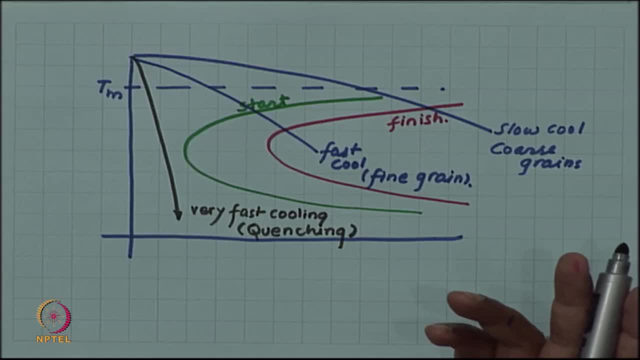 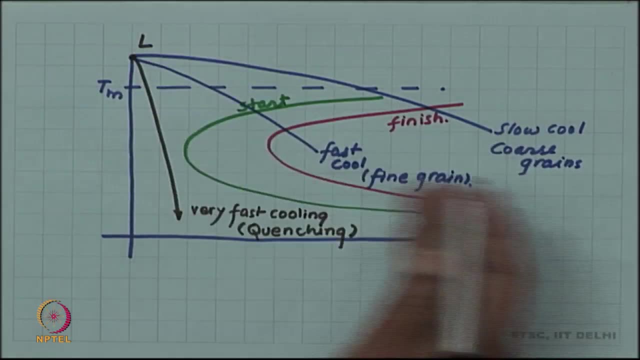 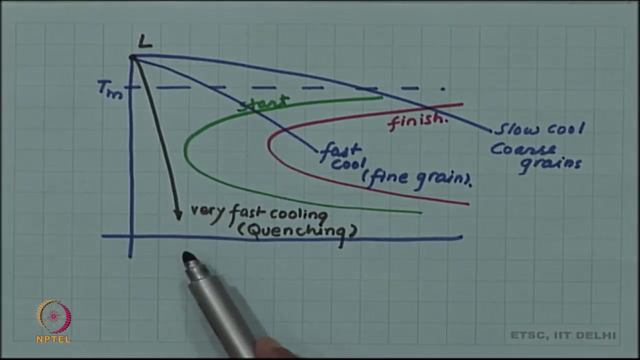 liquid. So what will happen? What will be the end product? So, obviously, since it is started with liquid, it started in the liquid phase and it is never transforming to the solid phase. that liquid continues to remain at lower and lower temperature. 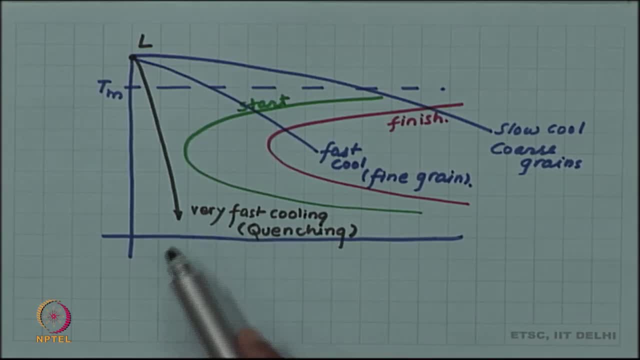 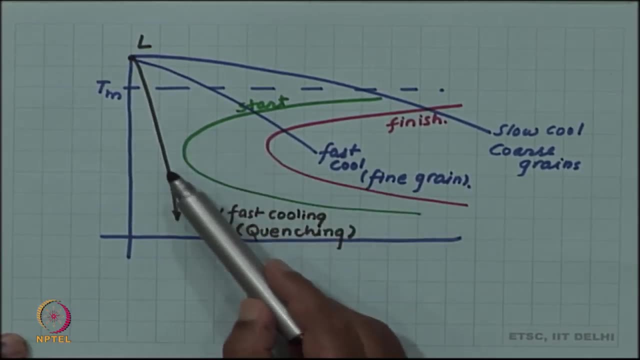 So, essentially, what you have is an undercooled liquid here. Okay, And this like, although it is not transforming into solid, its physical property keeps changing, and one of the physical property is the viscosity, So let us note this. So, transformation: 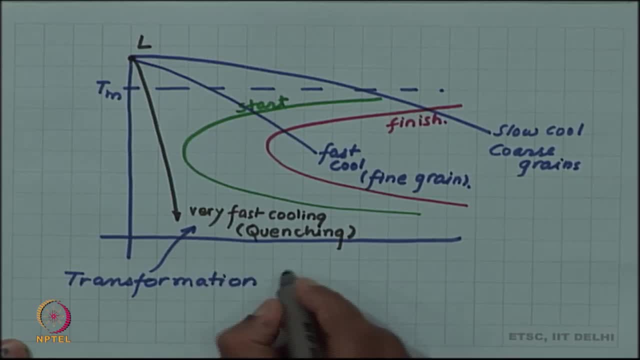 Okay, Okay, Okay to solid is suppressed, So you end up with undercooled liquid. However, as temperature falls, viscosity increases. This will mean that this liquid will become more and more viscous as the temperature is falling, So below a certain temperature, the liquid will. 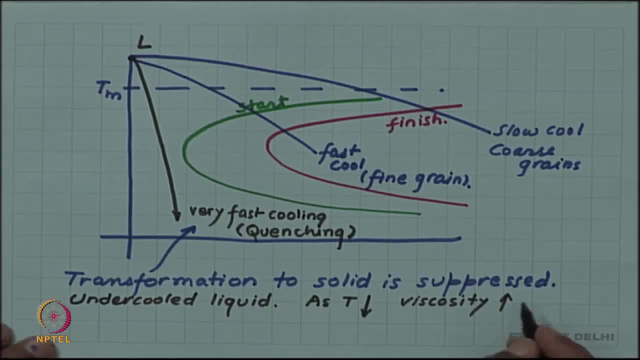 be so viscous that will appear like a solid. So, at very low temperature, viscosity has a value like that of solid And such undercooled liquid which appear to be solid in terms of their viscosity, in terms of their flow property, is what we call glass. So, essentially, we 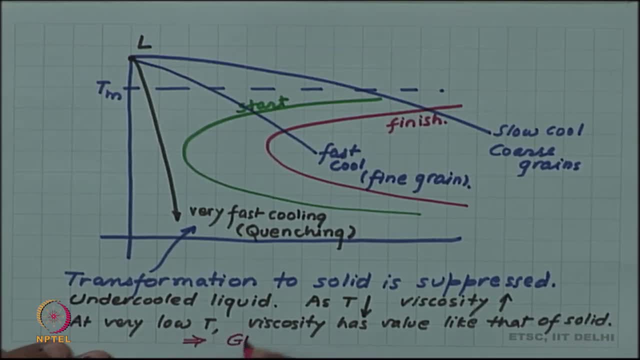 have formed a glass, which is also called amorphous solid. So very fast cooling or quenching curve is avoided. it never hits the start curve will then result in the formation of glass. So the TTT diagram for liquid to solid transformation also helps in understanding why very fast. 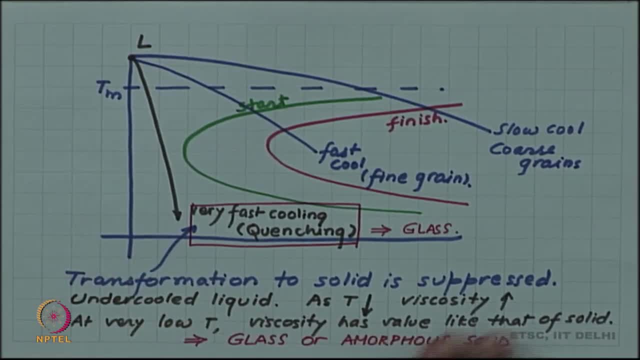 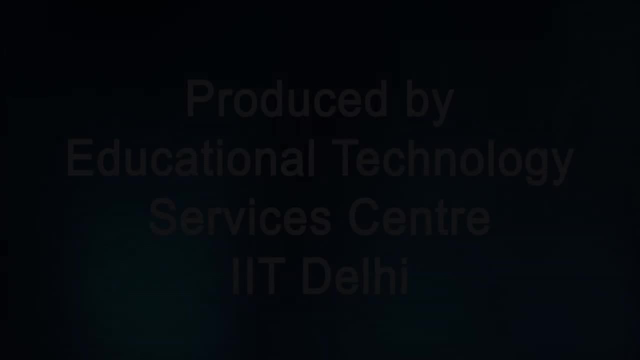 cooling can give us glass instead of a crystalline. solid Subtitles by the Amaraorg community.